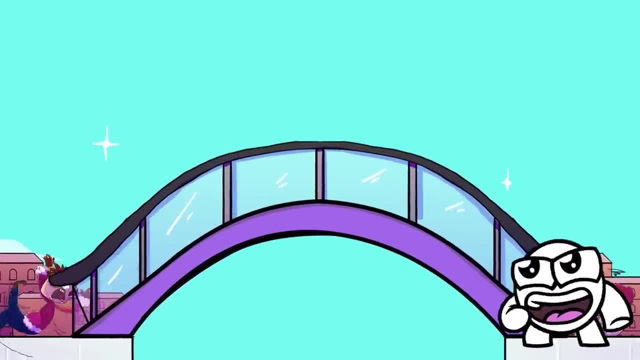 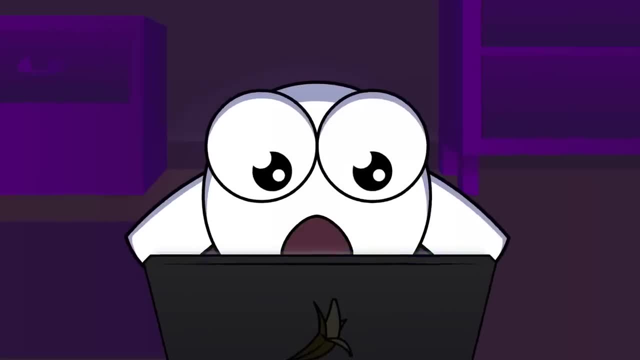 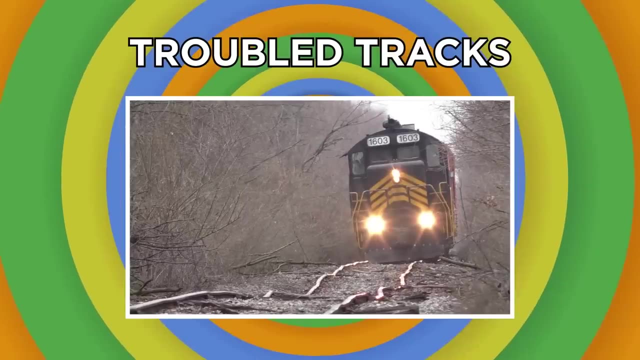 And when they do, they can be hilarious With that. let's take time to look at some of the funniest engineering fails ever. Troubled Tracks. What you're currently seeing is a train en route from Ohio to the town of Cecil on a. 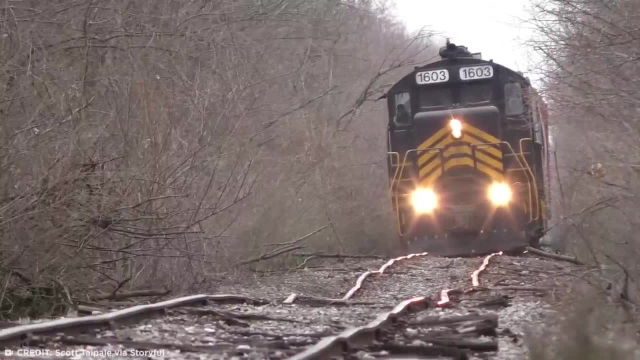 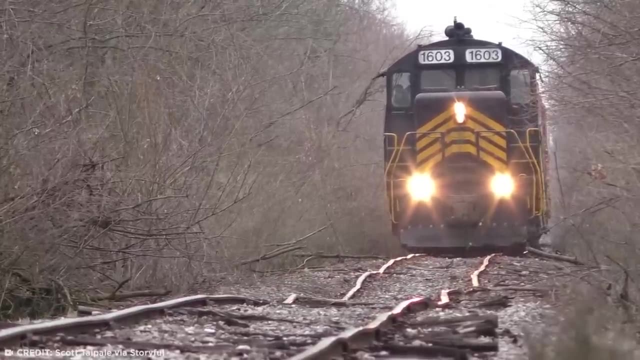 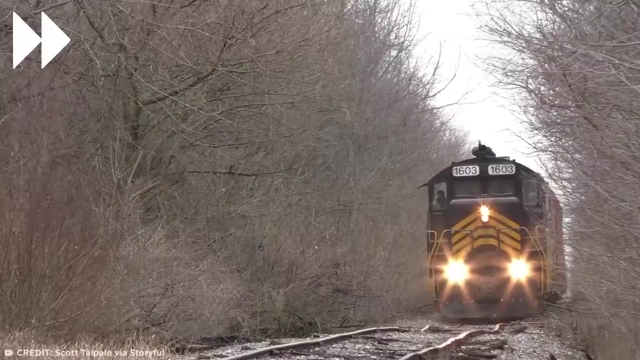 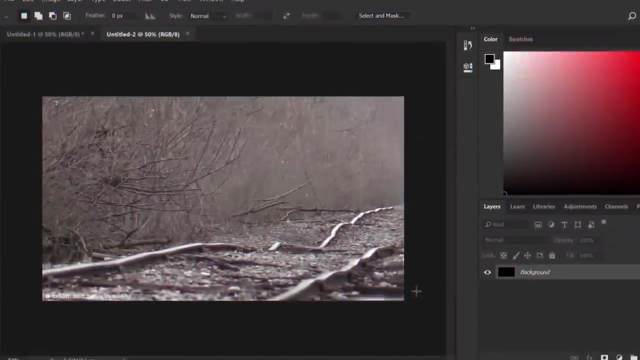 routine cargo delivery Only. instead of traveling along solid sturdy rails, the train precariously wobbles across tracks that look like they belong on a roller coaster, not a railroad. While it looks like a Photoshop trick, the melty tracks are a real, if unusual. 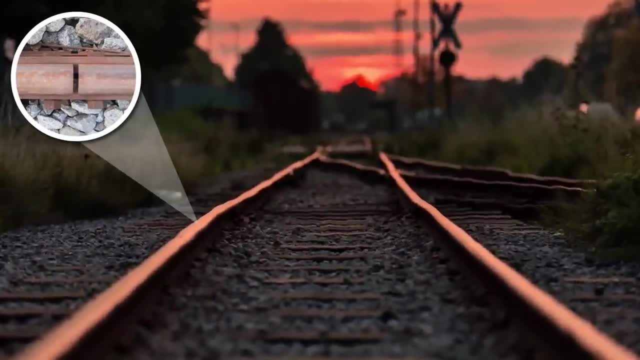 phenomenon. Prolonged heat is known to make metal relax and expand and then contract when things cool off. Usually this isn't unusual, but it's a high-tech way to get things done. Usually this isn't unusual, but it's a high-tech way to get things done. Usually, this isn't. 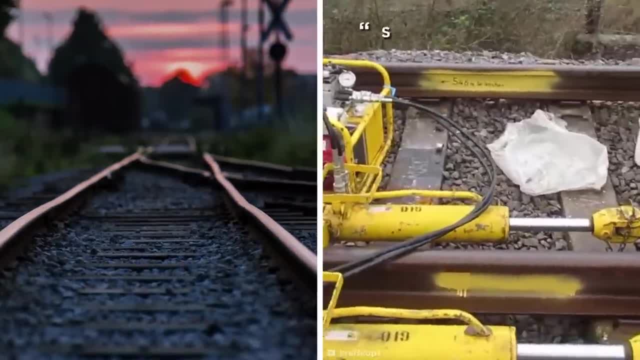 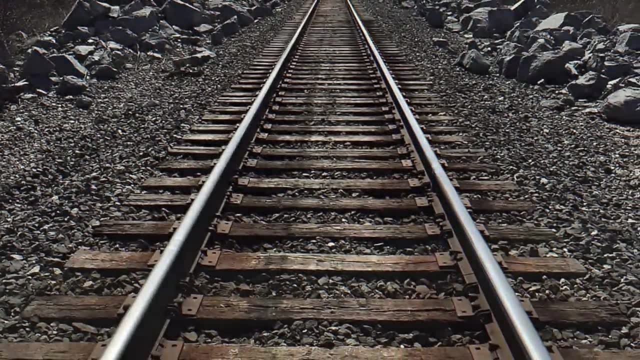 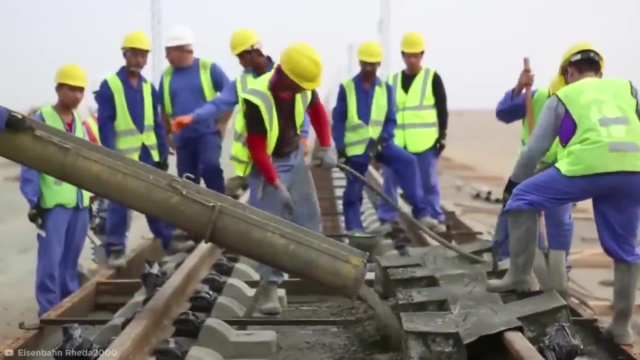 a problem for railways, as tracks undergo a process called stressing. This increases the temperature range most tracks can maintain their shape at and guarantees they return to their original shape if they do expand Hastily. assembled tracks that forgo the stressing process, however, 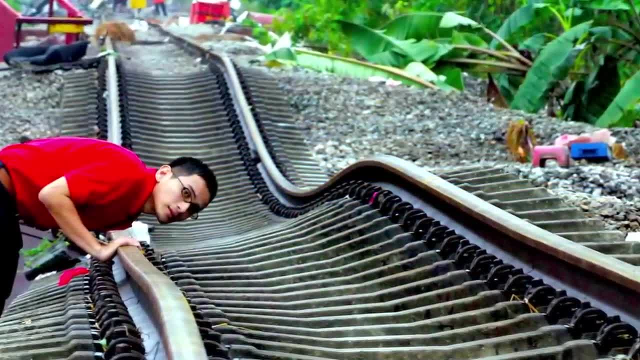 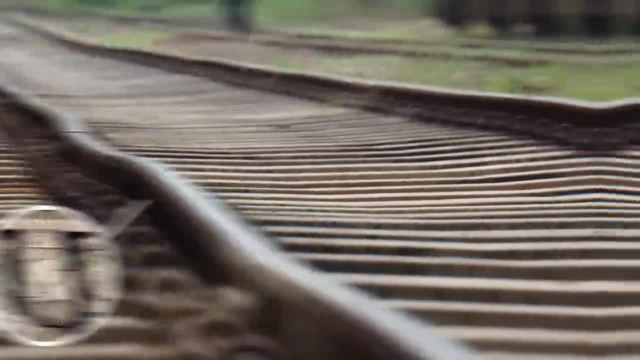 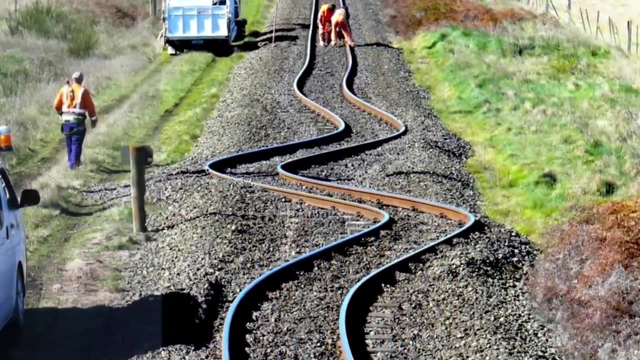 run the risk of the spaghettification we see here. This is when important ballasts become damaged or dislodged as the tracks expand, and when they contract they don't revert back to their original shape. These tracks in New Zealand likely only had a small weak point along the 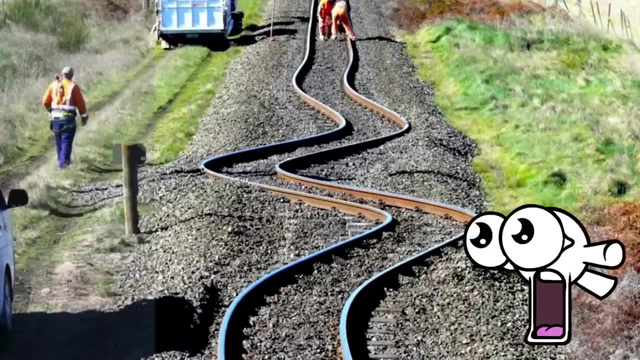 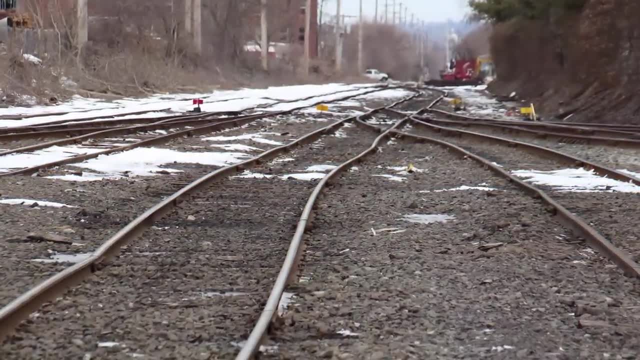 railing, but that was enough for them to become completely spaghettified when the region was struck by a 7.1 earthquake. So, despite looking tough, imperfect railroad tracks can be sensitive, And while many areas of the world don't have to worry about earthquakes, 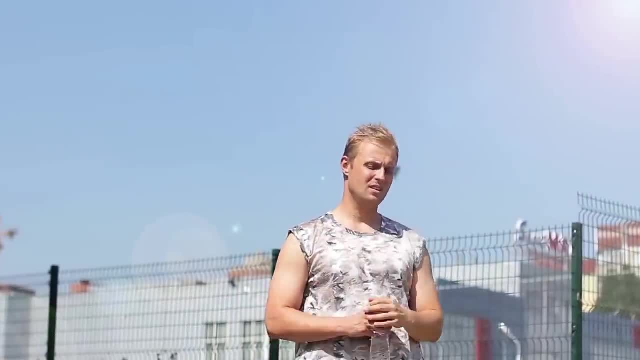 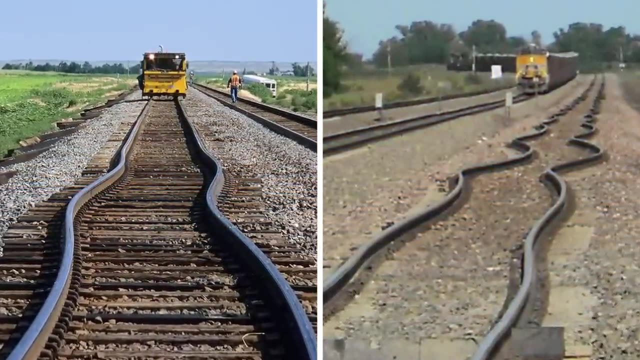 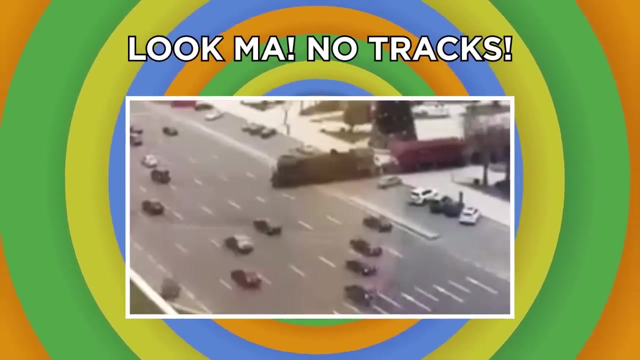 we all are. We all need to worry about rising temperatures as summers get hotter and hotter across the globe, potentially spaghettifying more and more train tracks. So I hope we all love roller coasters. Look Ma, No Tracks. Vehicles are pretty simple to understand: Cars go on the road, Trains go on the tracks, Not hard. 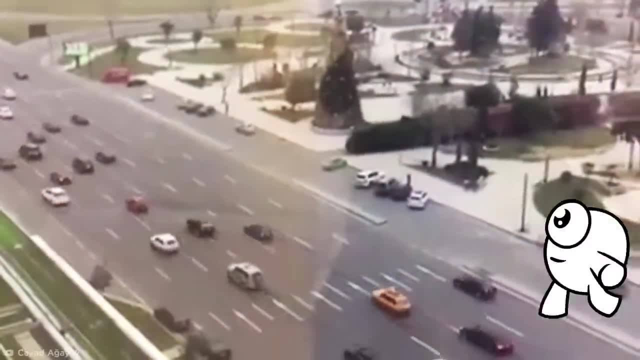 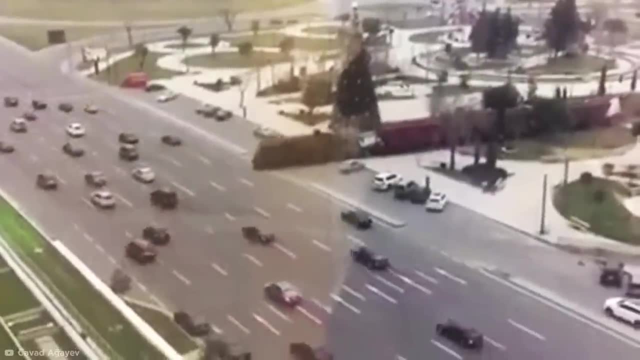 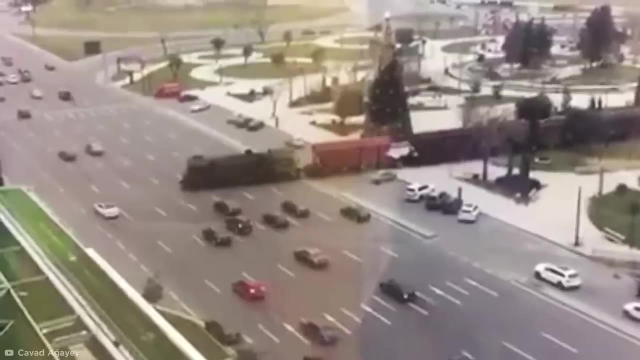 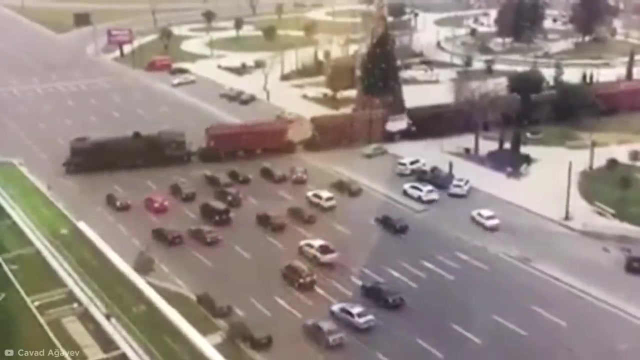 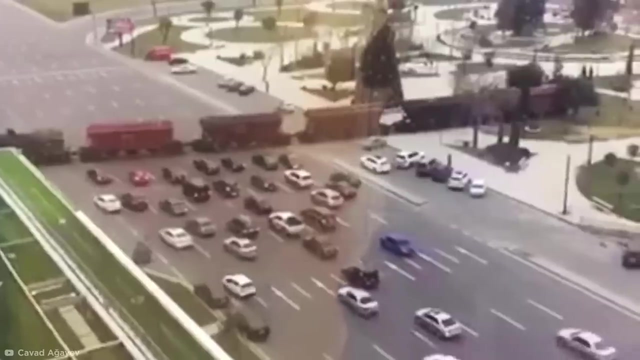 to wrap your head around, right, Except the engineer behind this mad design decided that this train would go on the road And that the train would go wherever it damn well pleased. So what you're looking at isn't a rogue train pretending it's a car. it's a train that would go wherever it- damn well pleased. 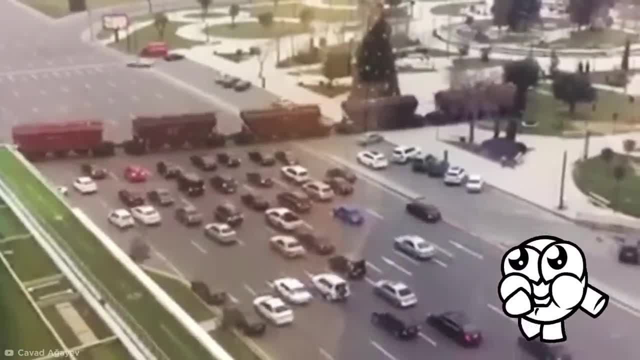 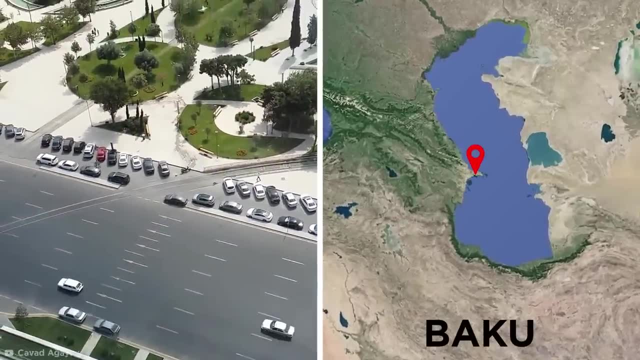 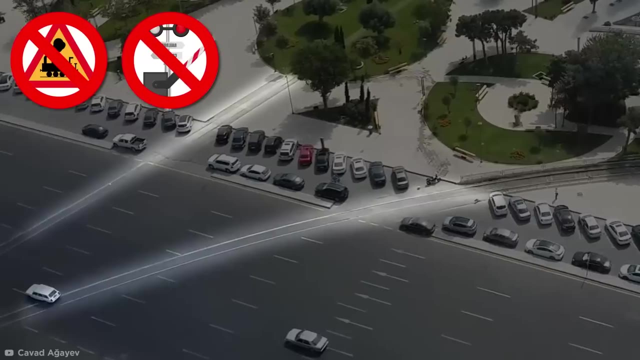 No, what you're looking at isn't a rogue train pretending it's a car. it's just terrible design. This highway was located along Neft Kalar Avenue in Baku, the capital of Azerbaijan. As you can see, there are no crossing signs, no barriers, and the tracks are nearly invisible. 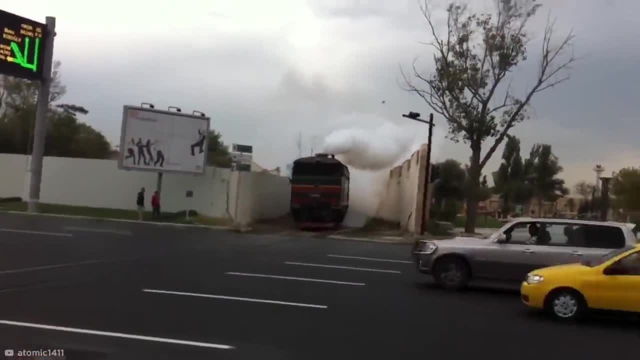 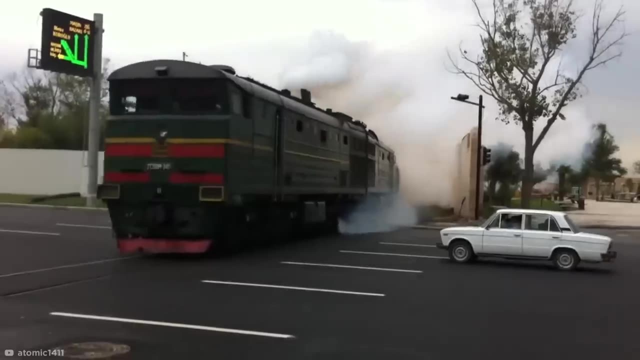 The only warning motorists get is a very desperate sounding horn from the fast approaching train. This woman's train track is peeking at his passenger. passenger, when he's in the middle of never images that a train is a train. Okay, who Was疑? sign nta. 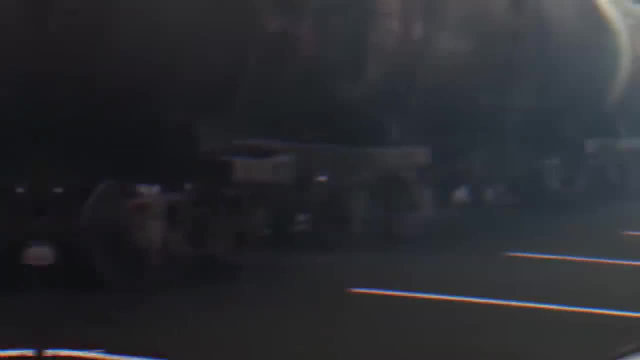 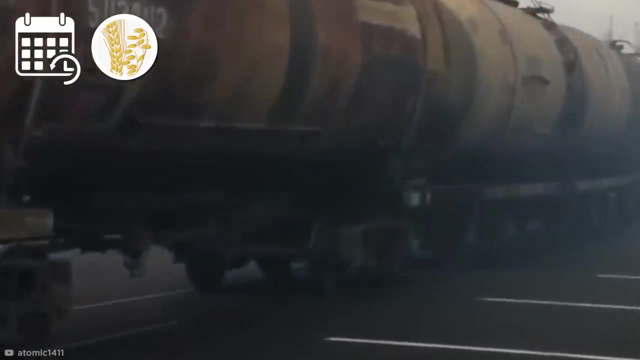 Okay. who, in their right mind, thought this was a good idea? Well, it would seem. the railway was built many years ago to transport the grain from the docks on Baku's Coast. The 7-lane highway was built over the tracks as the city developed. 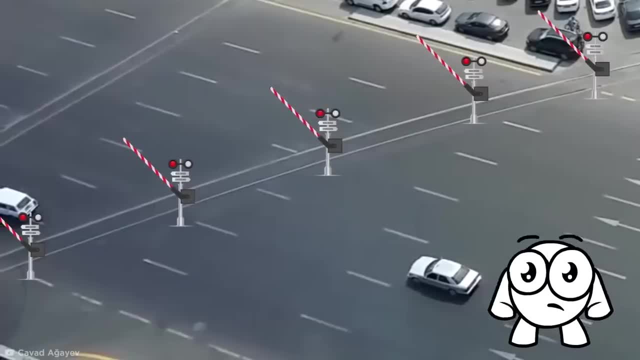 but the engineers didn't seem to think a warning system was necessary. Weird ¿¿¿¿¿¿¿¿¿¿¿¿¿¿¿¿¿¿¿¿¿¿¿¿¿¿¿¿¿¿¿¿¿¿¿¿¿¿¿¿¿¿¿¿ withdrawamp،. 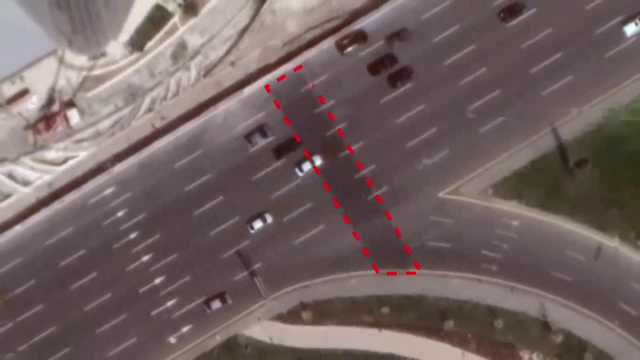 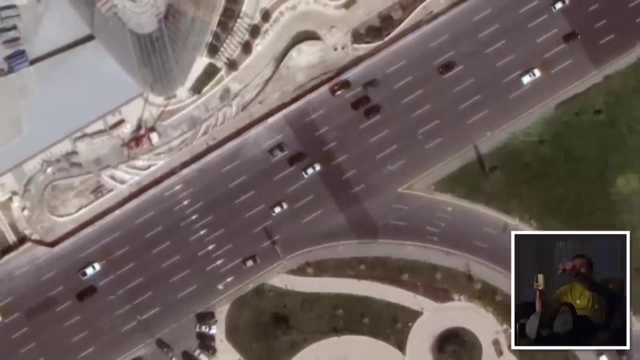 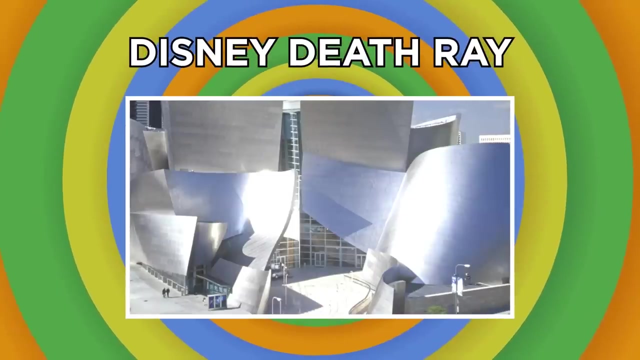 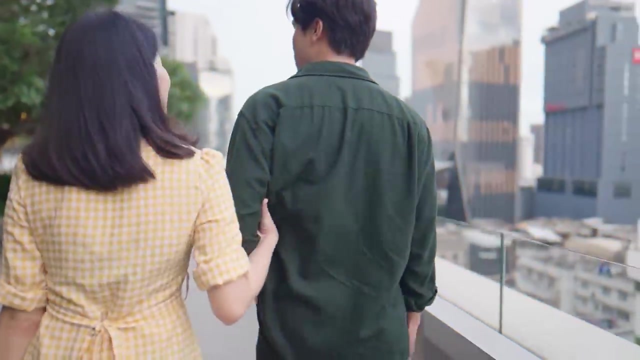 Regardless, thanks to ongoing development, tracks have since been tarred over, though you can still see proof they existed on Google Maps. Sorry, Baku, You can't hide this dangerous mistake from the rest of the world. Disney Death Ray Quick question: Where is the happiest place on Earth? The arms of a loved one. 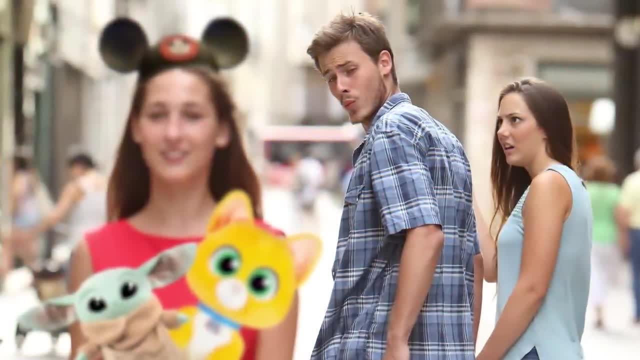 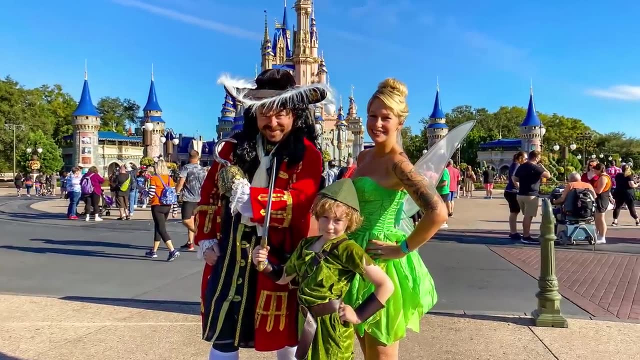 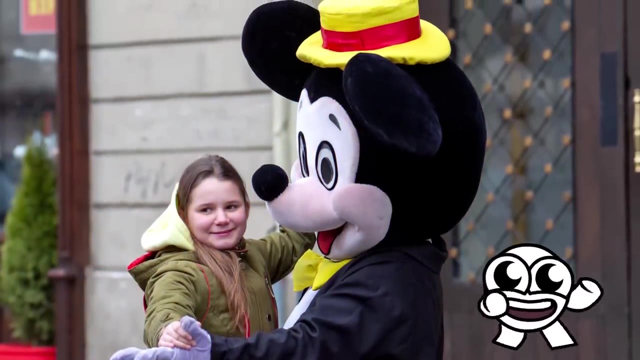 No, You can't buy merchandise in the arms of a loved one. It's Disney World, of course, the only place where adult men are encouraged to interact with kids in weird, identity-hiding costumes. Ah, happiness. Well, in 2003,, Disney decided to add a little more prestige to their name by commissioning famed architect Frank Gehry to design a classy new concert hall for them, To be located right in the middle of downtown Los Angeles. This was his final proposal: Sleek, futuristic and kind of trippy. Obviously, the unconventional design split people's opinions. 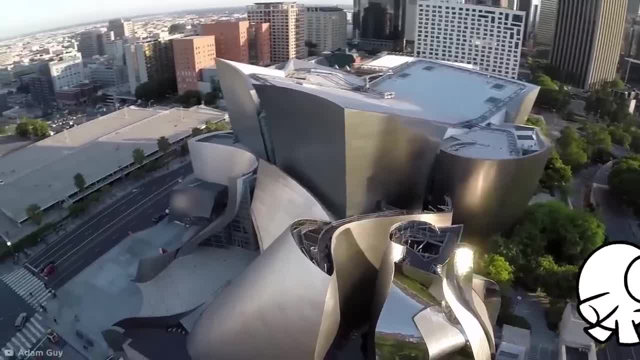 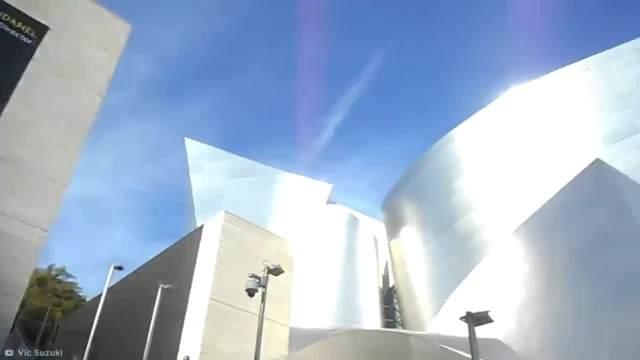 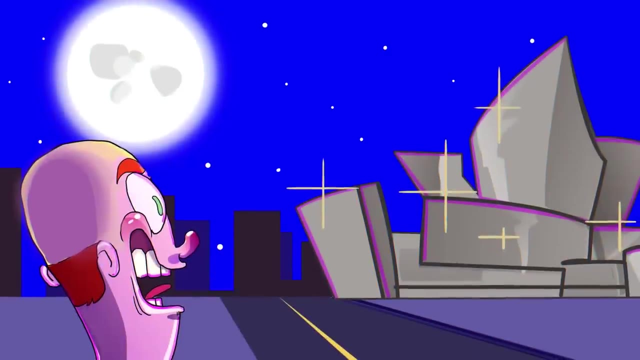 Though it's clearly an impressive piece of architecture, it's also a bit of an eyesore in more ways than one. You see, this metal abomination was comprised of over 12,500 curvy stainless-steel panels. This meant that, while you could safely appreciate the concert hall's unique design at 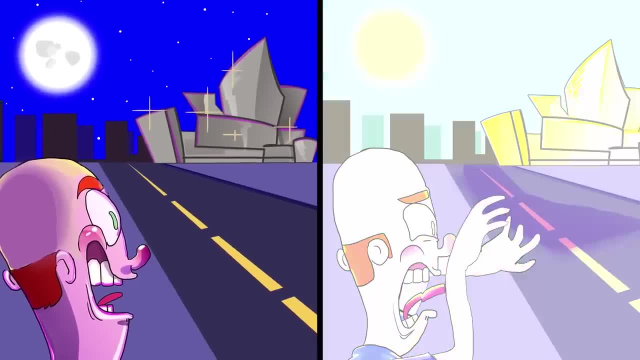 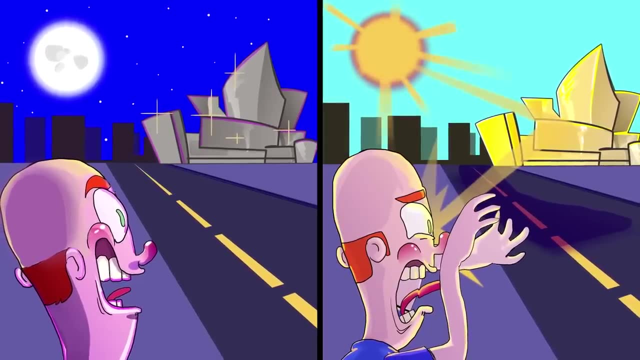 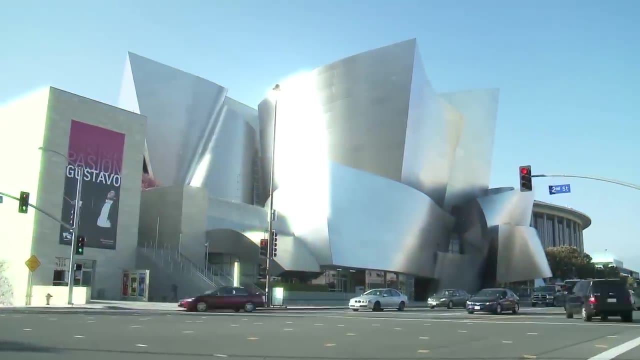 night. during the daytime it became blindingly bright. The steel panels covering the building were extremely reflective, to the extent where people said looking at the building in the day was like staring directly at the sun. To make matters worse, the hall is right next to a major 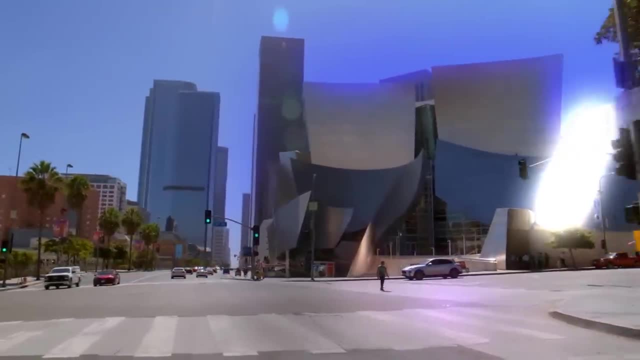 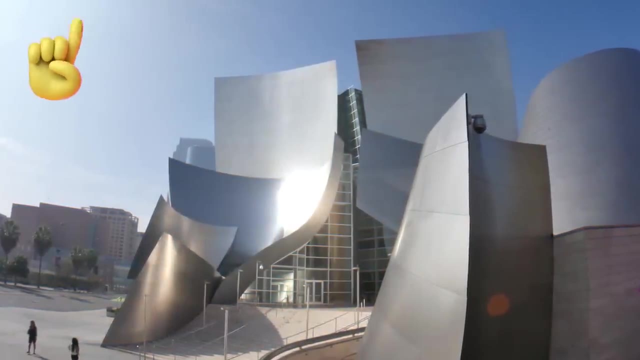 road and its unavoidable glare was responsible for the building's appearance. In the end, the hall was responsible for temporarily blinding multiple drivers. But wait, there's more. You see, the concert hall didn't just reflect light, it also magnified heat. 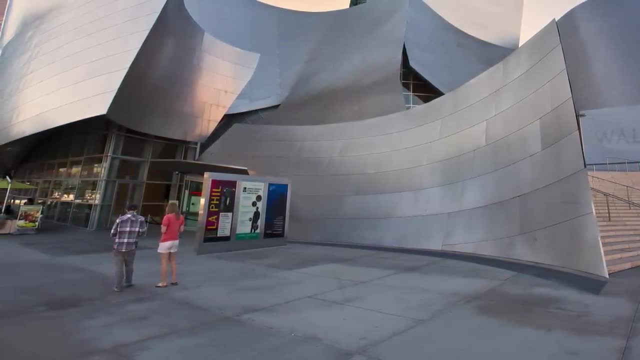 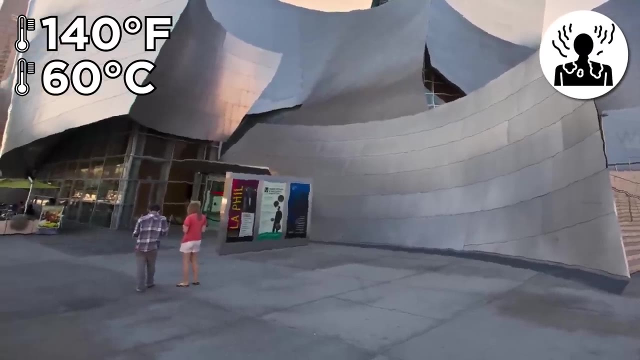 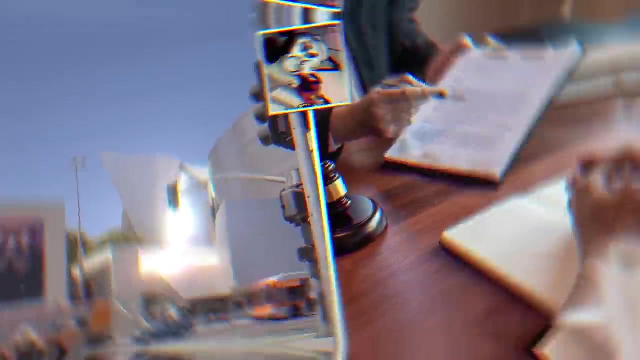 According to some bystanders, the sidewalk around the metal monstrosity could get as hot as 140 degrees- enough to leave some serious burns if you weren't careful, Realizing they had basically installed a permanent lawsuit machine. Disney acted fast. They had. 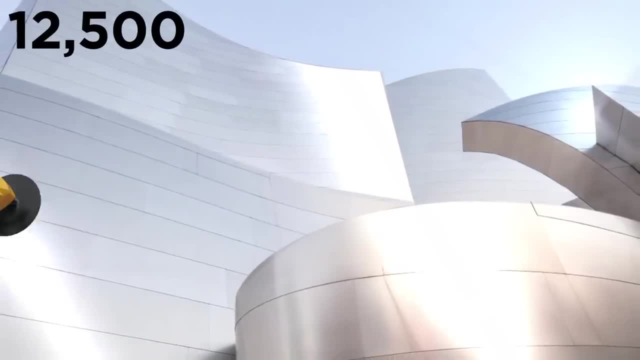 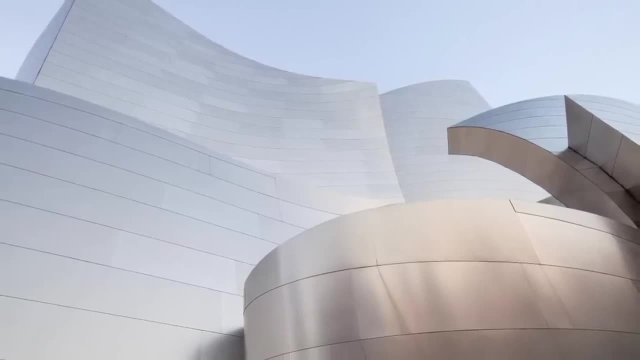 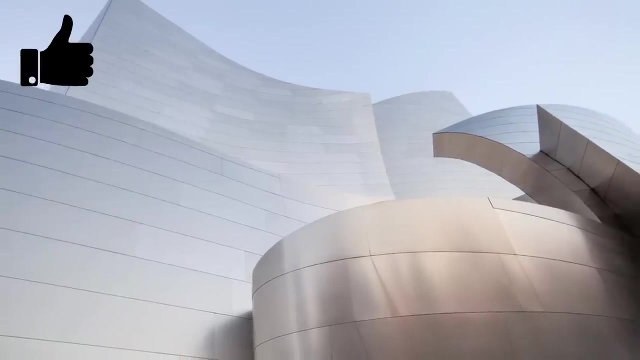 each and every one of those 12,500 panels sanded down, making them significantly less shiny. While this means the building isn't quite as grossly incandescent as Gary envisioned it, it's a heck of a lot safer. Good thing, too, because after Disney bought the rights to the 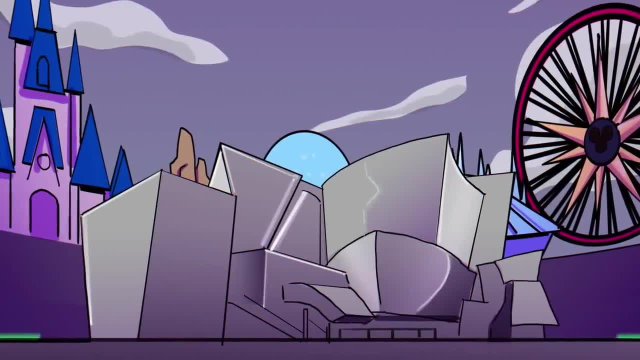 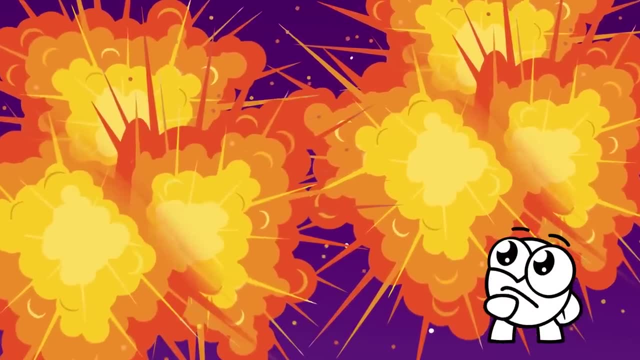 Star Wars franchise in 2012,. that super-scorching light beam would have made it look like the concert hall was Disney's homage to the Death Star. Hmm, I wonder if they thought about aiming it at Universal Studios Tread carefully. 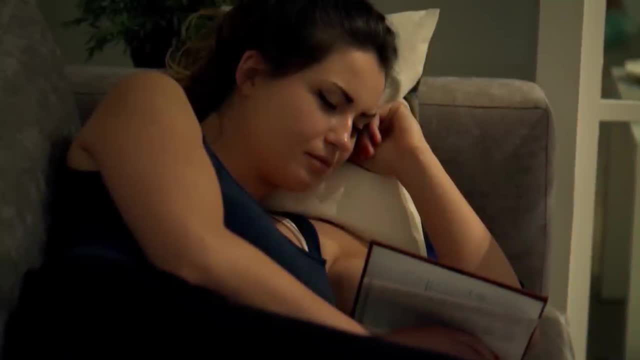 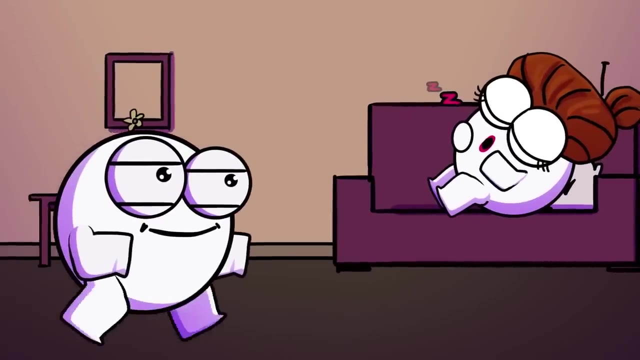 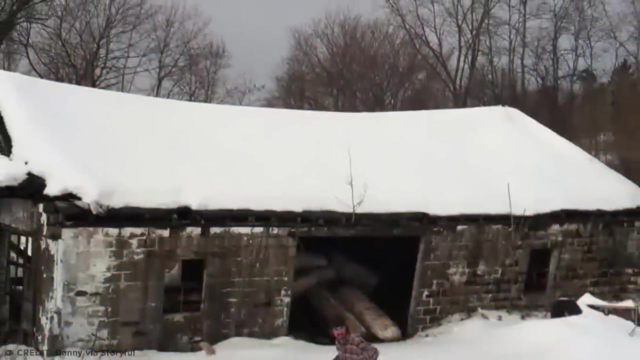 Have you ever come home to find a loved one fast asleep and begun creeping around the house like a spy so as not to wake them up? I have a few times, but thanks to my two left feet, it usually ends up with me waking up, Mrs Amazed. Still I can breathe a sigh of relief, knowing my loud footsteps. 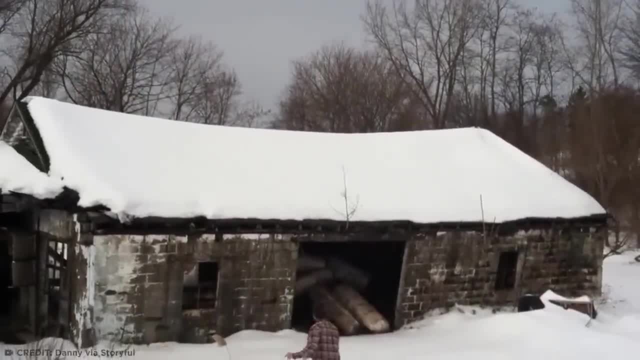 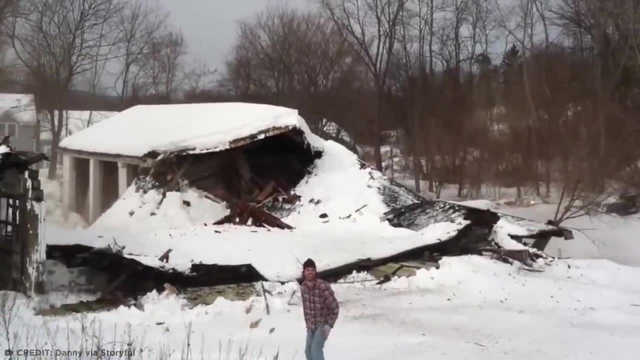 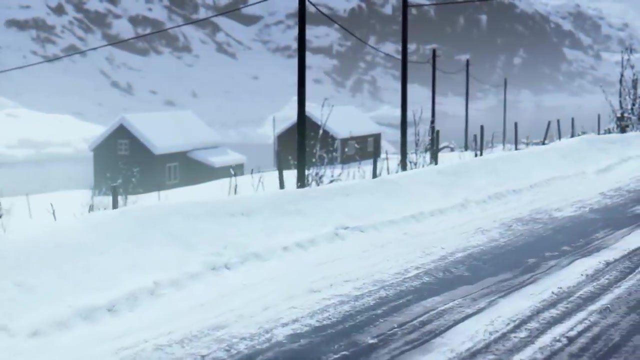 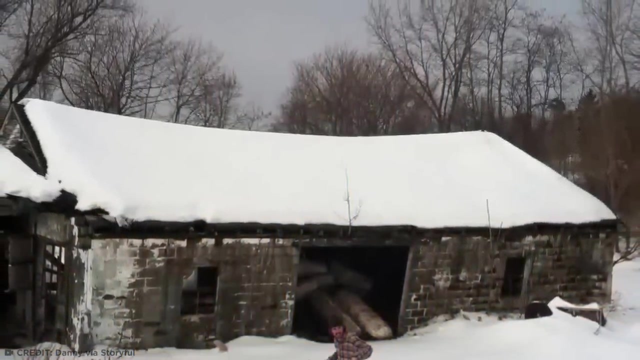 have never caused as much damage. Here's this. guys Dang Daniel Johnson and his brother from Pauling, New York, were out exploring some scenic winter wilderness when this old house caught their eye. Unfortunately, it seems the house's foundations weren't quite up to carrying the weight of all that snow. 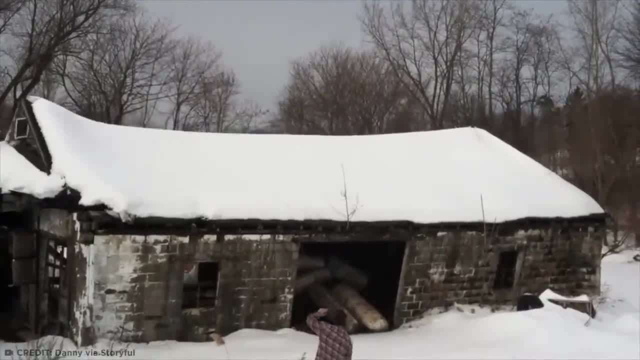 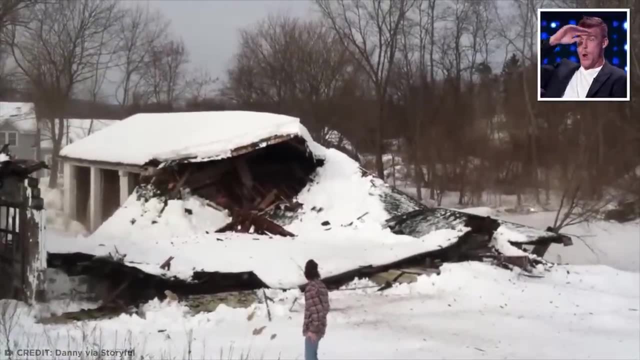 so a little jump was all it needed to jolt the structure and make it come tumbling down. Good thing he wasn't inside, or he'd have learned how hard it was to carry all that snow too. You know what's not hard, though: Hitting those like and subscribe buttons down below. 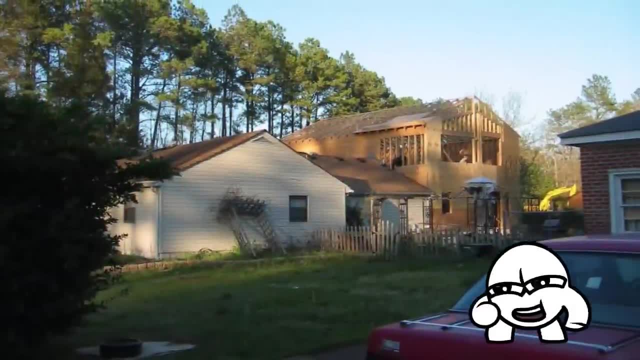 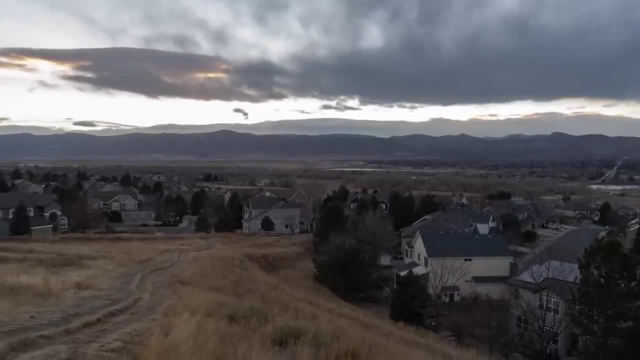 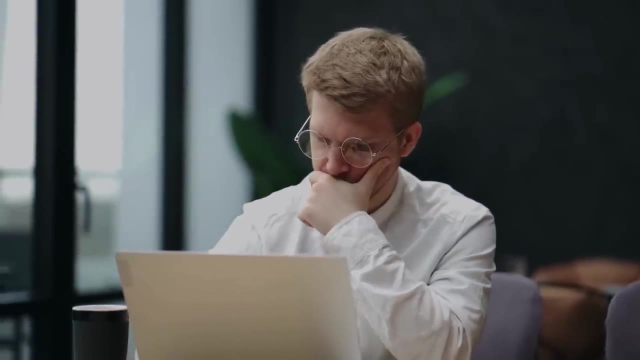 They're so well-designed. Unlike this next funny failure, The House That Grove Built, Our next story takes us back to 2006 and onto the something-awful forums. If you've been on the internet a while, you're already holding your breath. 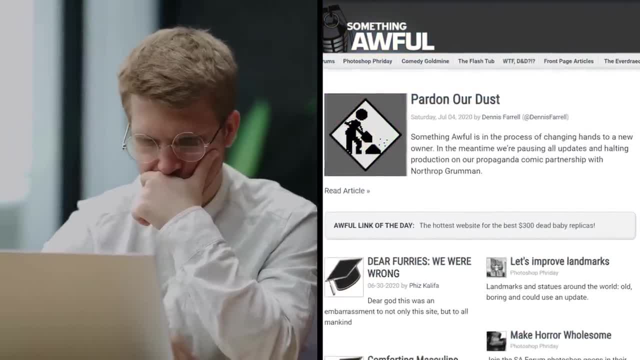 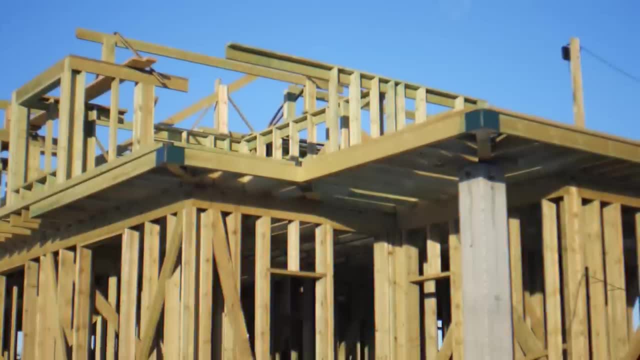 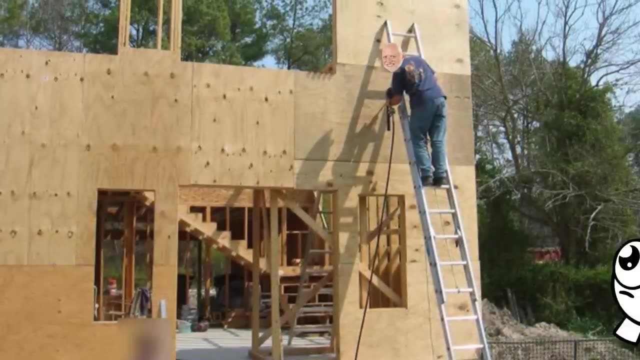 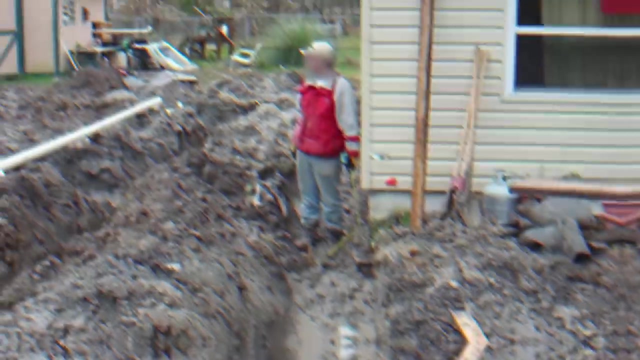 Our tale begins when a moderator for the forums by the name of Grover decided he was going to build his own home based on an MS Paint mock-up and, despite being completely unqualified, A perfect storm Users let him know this was a terrible idea, but Grover didn't listen and soon. 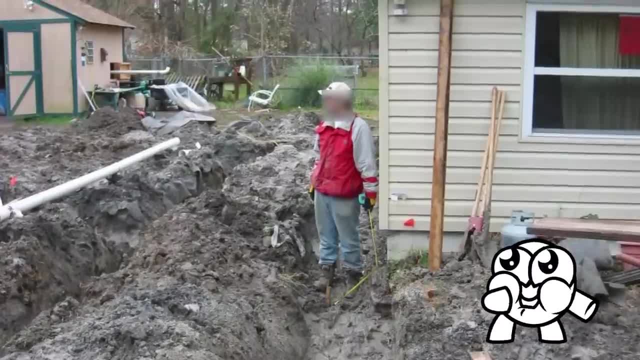 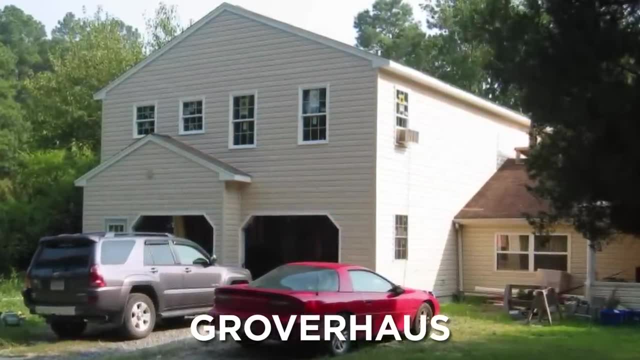 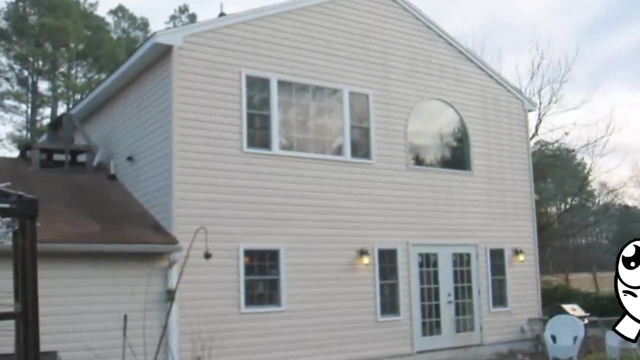 found himself the architect of the single most mean-looking house in the world. The house was named Building on the Planet, Grover House. Grover House really was the home that kept on giving. with each image, Grover posted telling a different hilarious story. Grover's um. 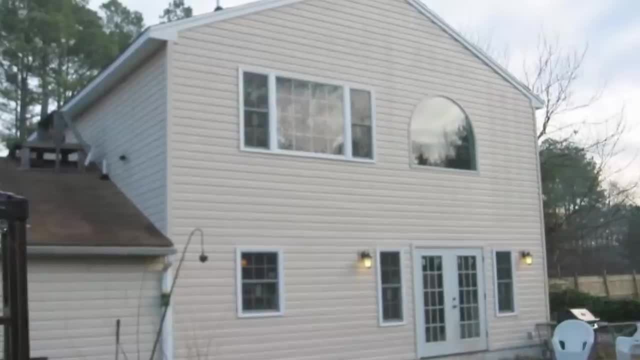 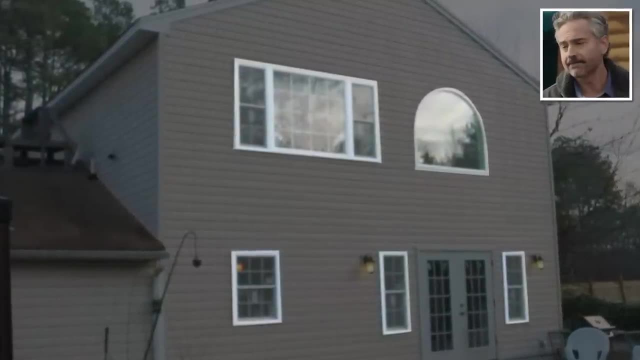 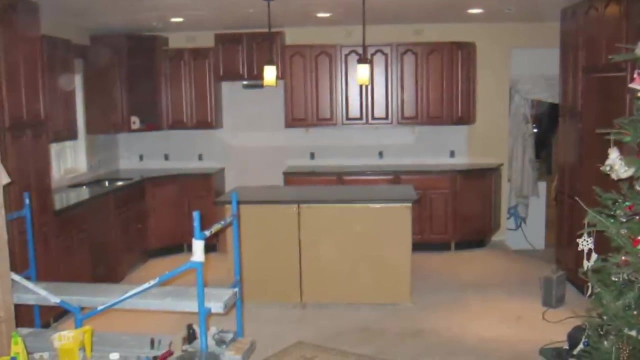 unique eye for aesthetics are on display here, where you can see seven windows in four different styles, none of which mesh together in a coherent way, And if you think they make more sense from the inside, they don't, Then there's this picture of his kitchen, which reveals that Grover thought 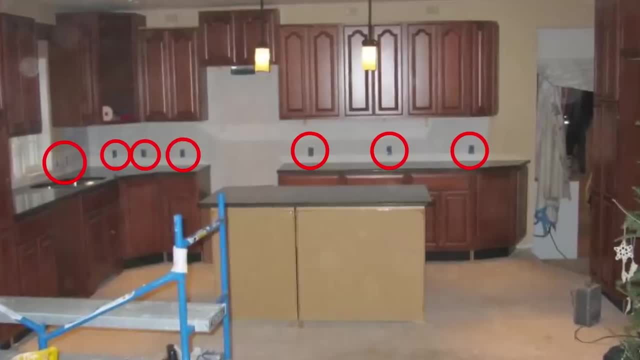 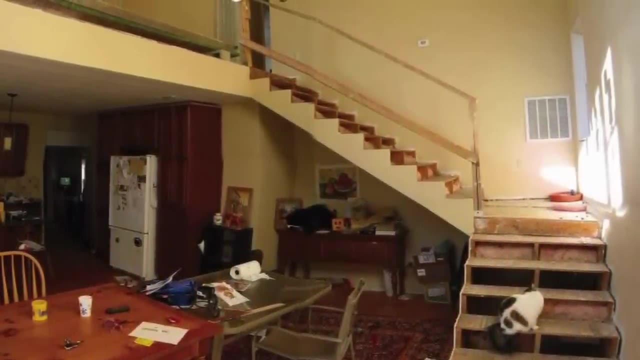 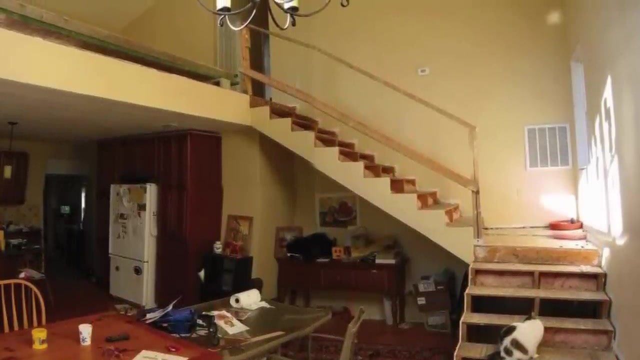 he would need eight power outlets, a foot apart from one another. Personally, though, I'm a fan of this picture of the interior, which reveals a window perfectly placed so that, if you fell down the stairs, you'd also crash through the window into a swamp below. Oh, did I not mention? 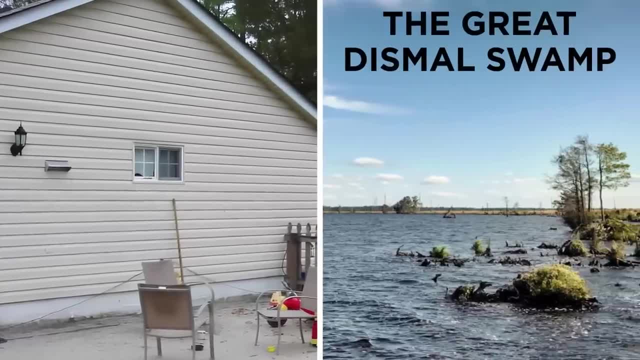 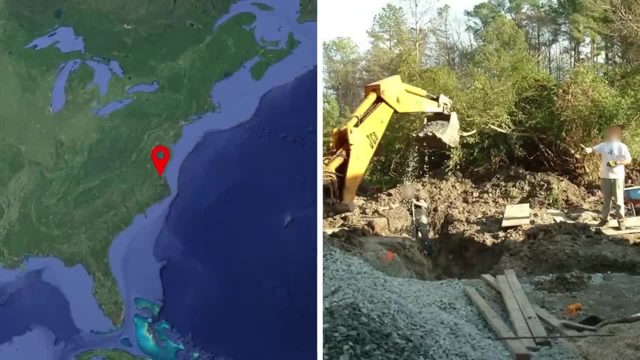 this entire house was built in a place called the Great Dismal Swamp. No, that's not an area in a Dark Souls game. It's a real swamp in Virginia that Grover thought would be the perfect place to build a home. Now, the funny thing about houses, though, is that they 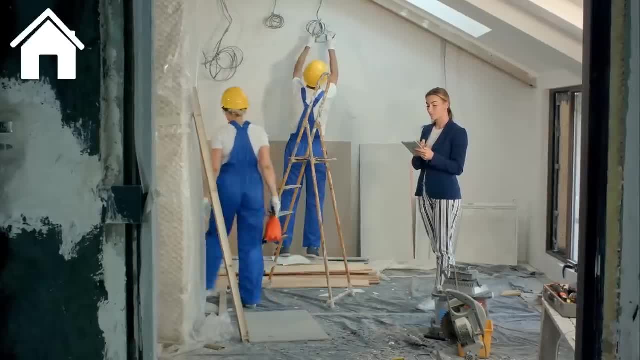 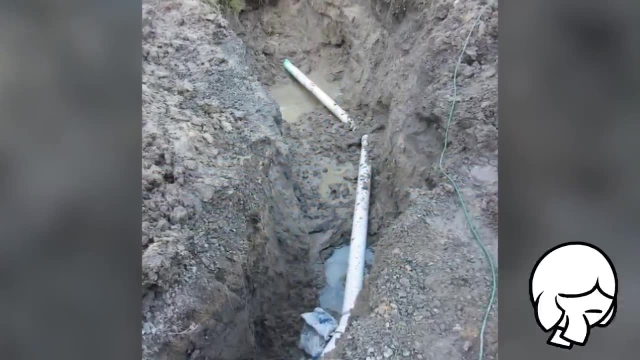 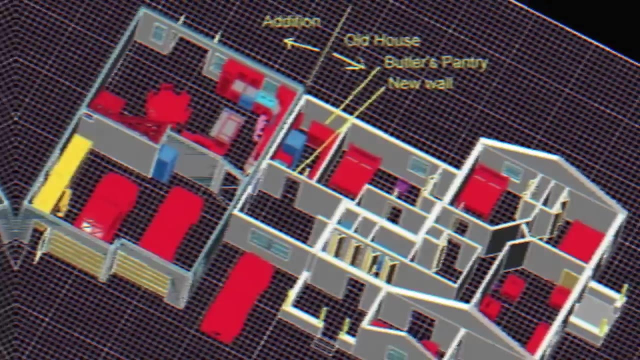 need to pass several safety inspections to be deemed livable. Well, as you can imagine, Grover House did not pass the safety inspection. This was perhaps due to his septic tank not being enough to support the waste his family would produce, or the fact that he was not able to. 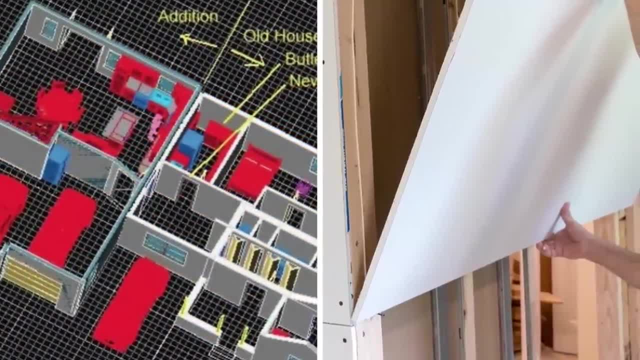 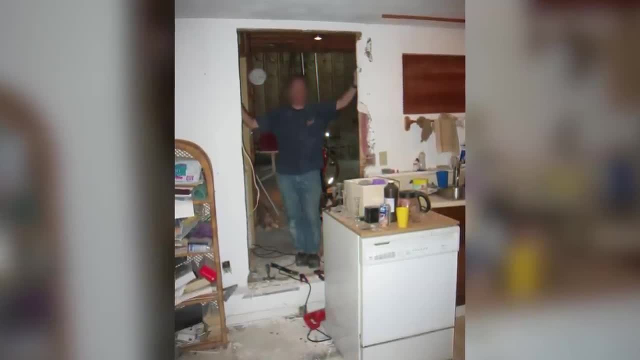 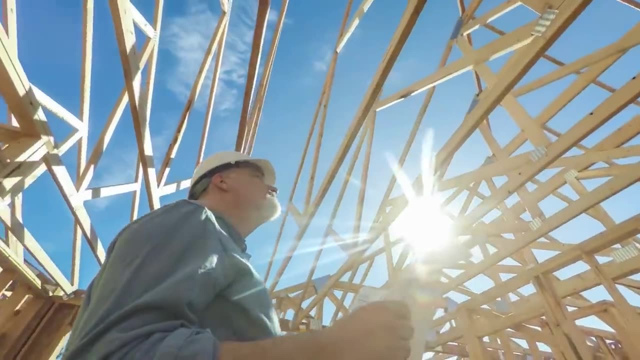 use drywall, a notoriously flimsy substance, as a load-bearing material. So Grover was finally forced to admit enough was enough and pack the whole thing in. Yeah right. Instead, Grover decided to become a qualified health and safety inspector, just so he had the authority to pass. 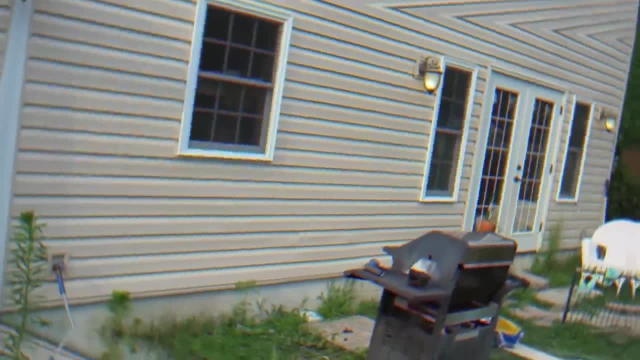 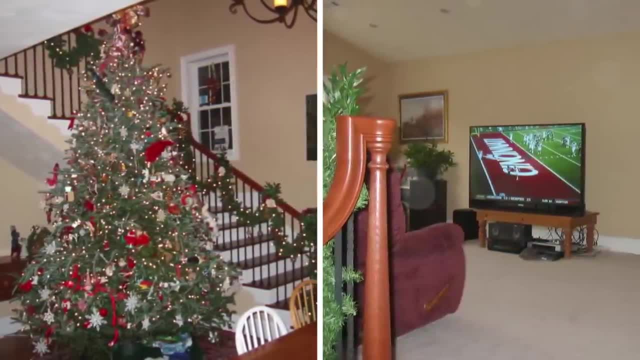 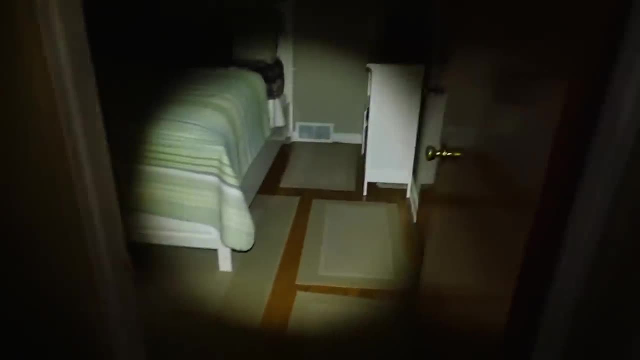 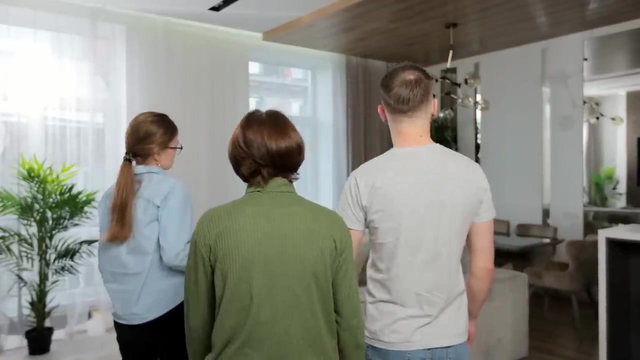 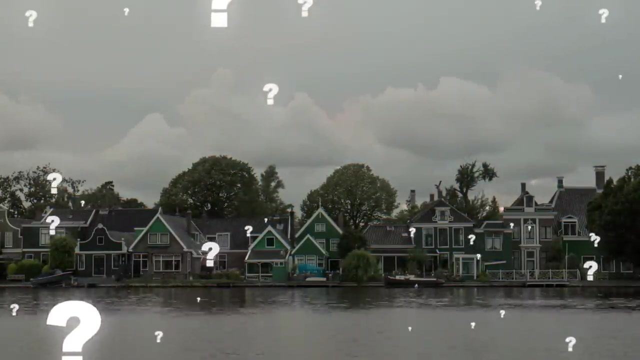 Come on Hollywood. where's our Grover House horror movie, Thirst Trap? If you've ever been house hunting, you're already aware that waterfront properties tend to be crazy expensive. But how close is too close? How about this house? Oh my gosh. 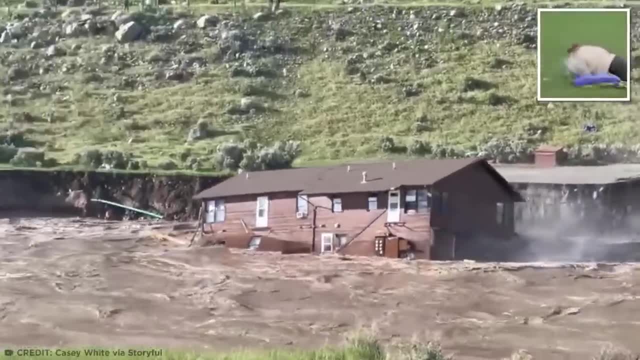 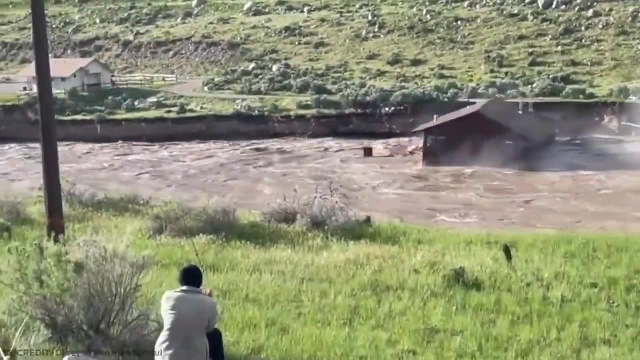 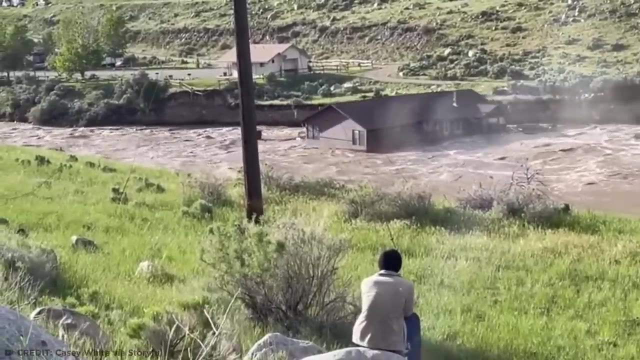 Dang And I thought my belly flop was impressive. This house was on the bank of a river running through Yellowstone, Wyoming, when it plummeted into the drink and was swept away by a mighty current. Luckily, no one was injured, as everyone had safely evacuated the house long before it. 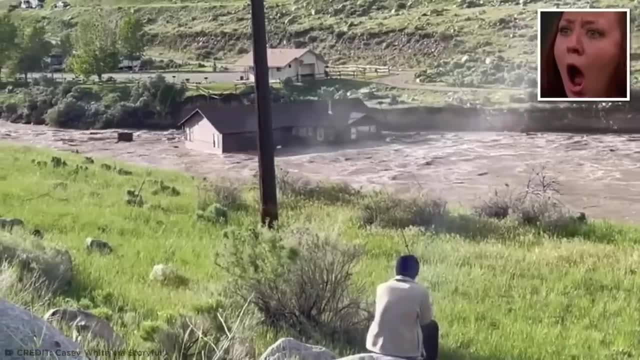 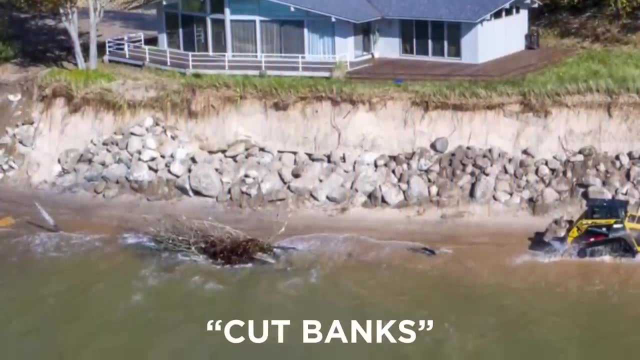 crumbled into the river. Though it's a crazy story, it's not a story that I want to tell. It's a story that I want to tell. This kind of thing happens all the time when houses are built along cut banks, which is to say, banks that have sudden drop-offs into bodies of water. 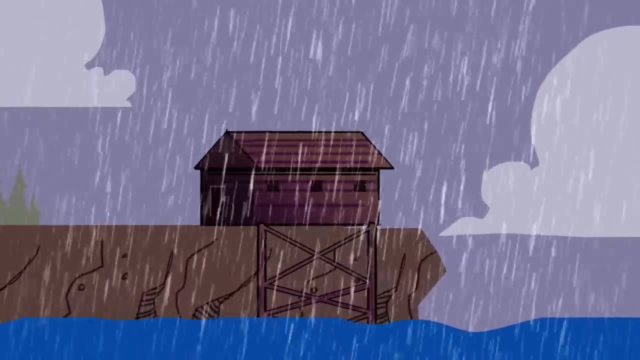 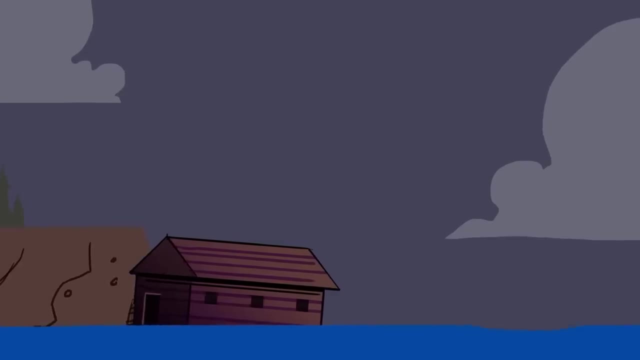 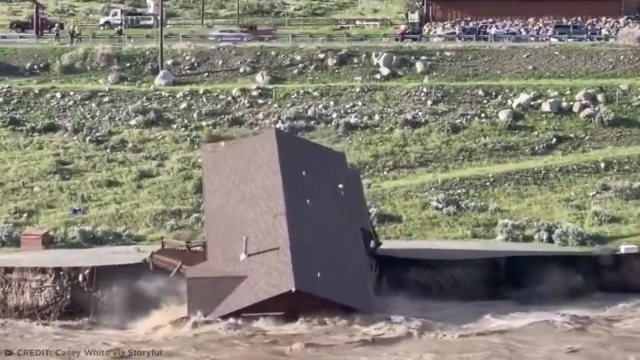 Because cut banks are exposed to the elements, they're particularly vulnerable to erosion. This means that with enough heavy weather, it's only a matter of time before your waterfront property becomes a water-logged property. Either that or this house was just real thirsty. 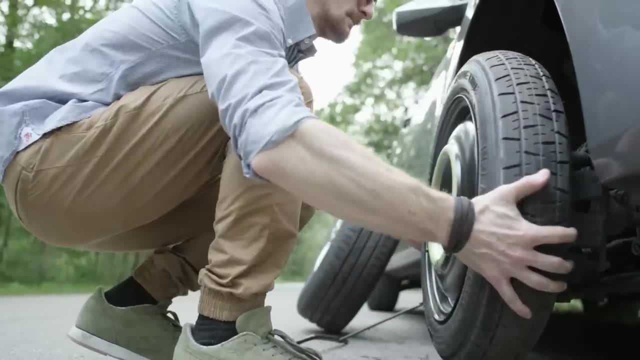 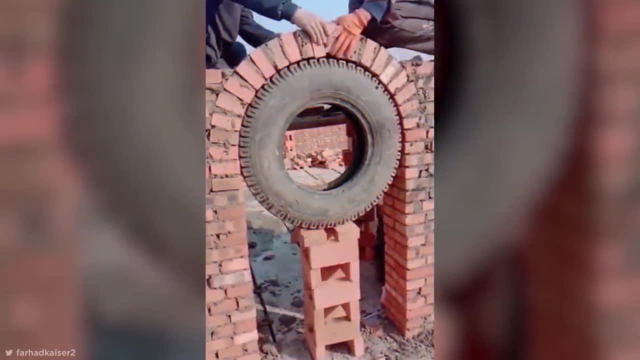 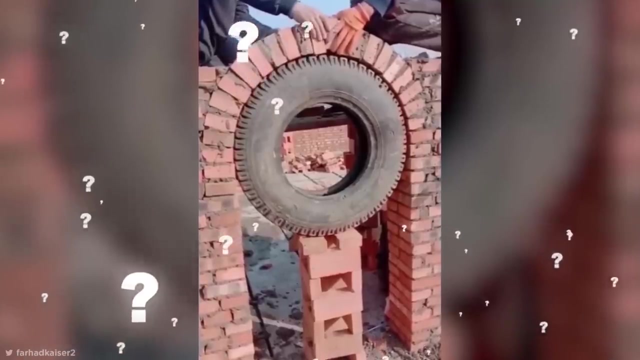 Tiring Work Pro-tip: Always make sure you have a spare tire on hand. After all, you never know when you might get a flat or uh need to embed it permanently into a construction site. It always pays to be prepared, I guess. So how did this tire end up here? Well, it may look like these builders were. 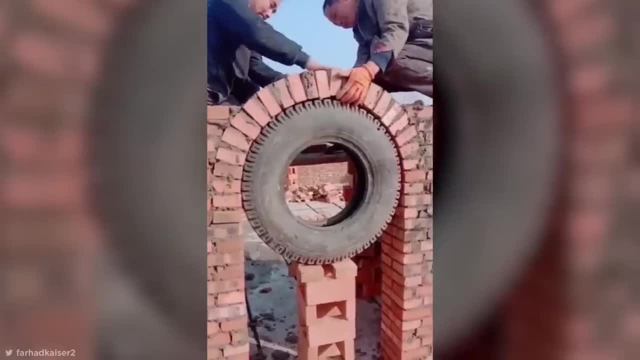 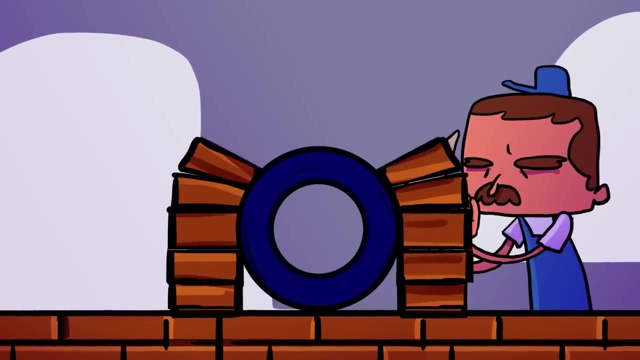 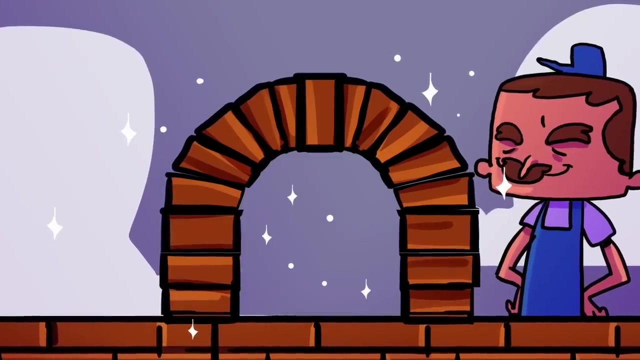 on autopilot and accidentally entombed a nice tire into their wall, but it's there intentionally. You see, the tire actually provides the perfect curved shape and foundation for creating a beautifully symmetrical arch, after which the tire can be removed. These folks may be constructing a simple archway. 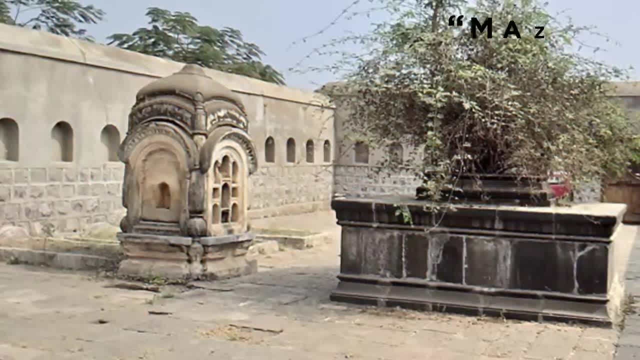 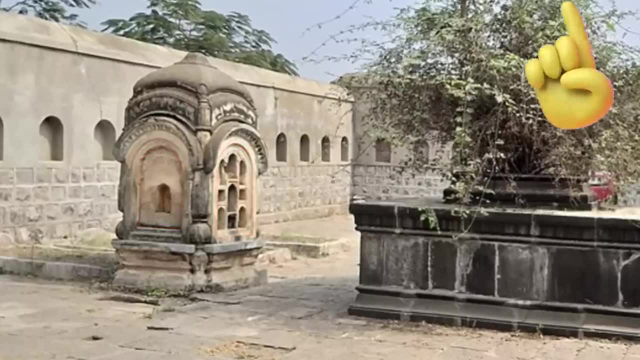 but it's so low to the ground. it could also be a mazar, which is a mausoleum or burial site consisting of a series of arches. This technique isn't strictly limited to austere tombs, though. Here we can see some civil engineering students in Ethiopia. 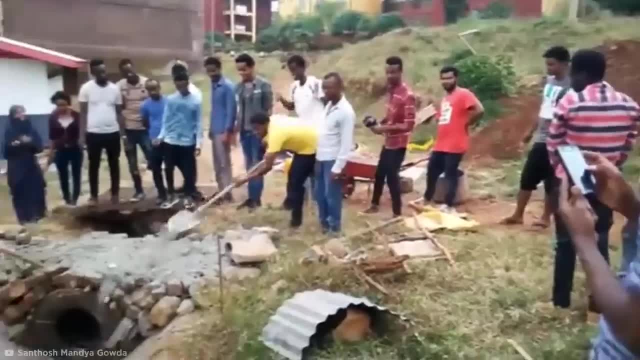 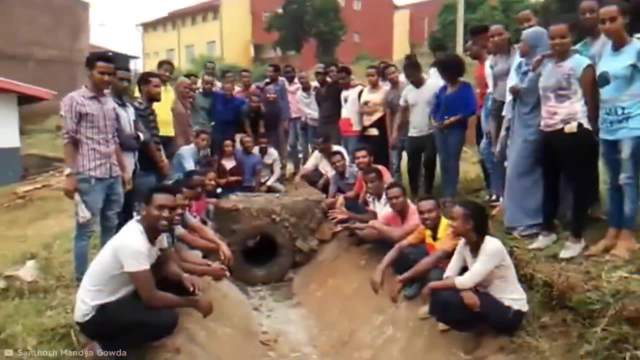 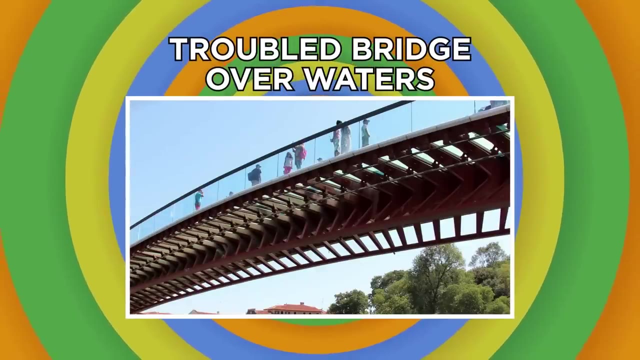 tasked with constructing a small arched bridge out of local waste. As it turns out, a leftover tire proved to be a great foundation. Talk about arch deco, Troubled Bridge Over Waters. Ah, Venice, A city of history, culture, canals and cranial injuries. 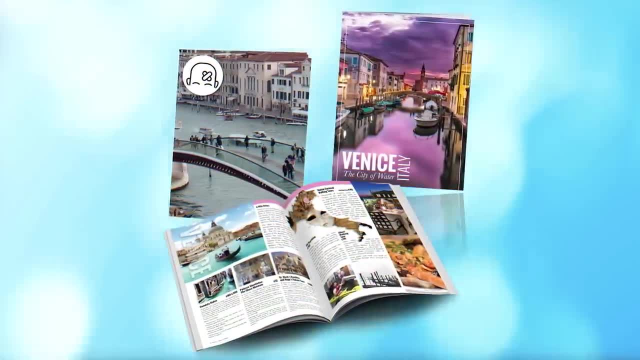 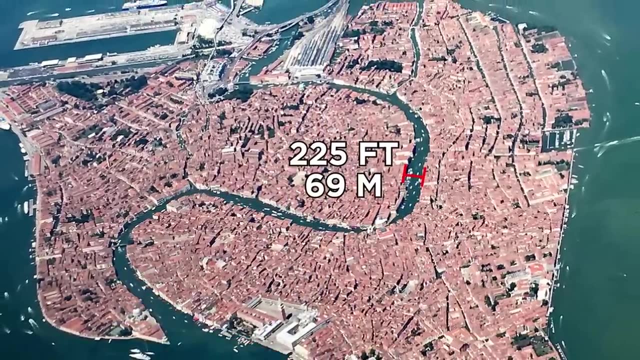 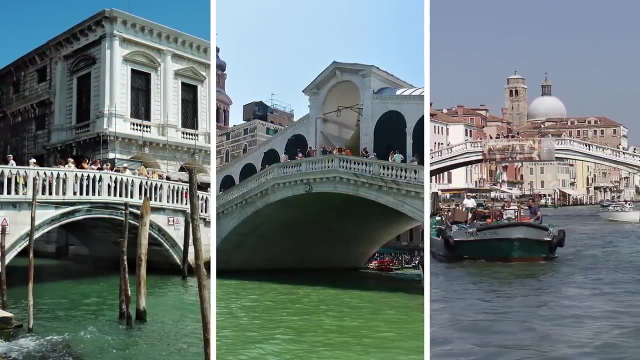 Surprised by that last one. Yeah, they tend to leave it out of the travel brochure. The city's impressive Grand Canal is over two miles long and 225 feet at its widest point. Despite this, however, in the mid-2000s there were only three bridges crossing it, which could get pretty. 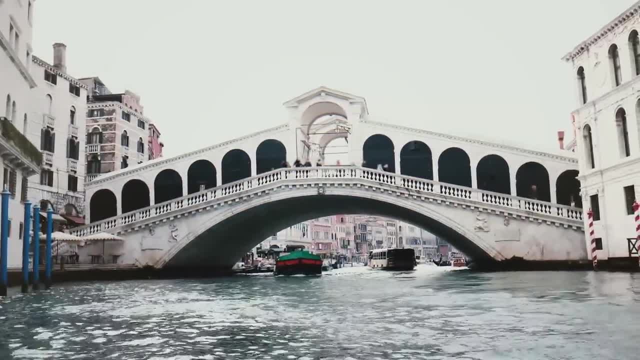 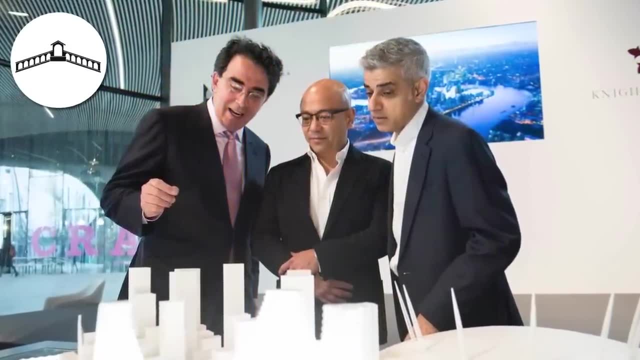 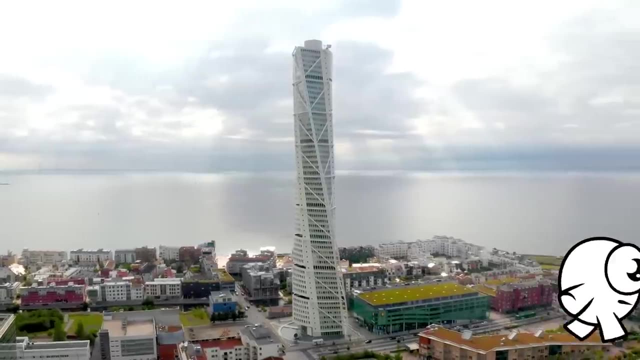 crowded. So in 2008,, the city commissioned famed architect Santiago Calatrava to design its fourth Grand Canal bridge. Calatrava was previously responsible for such eye-catching architecture as Sweden's Turning Torso Tower and Spain's Auditorio de Tenerife. 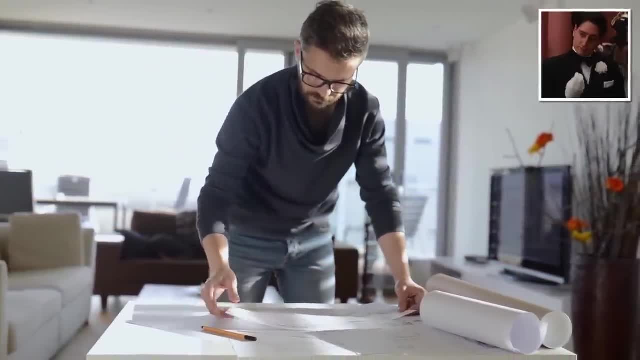 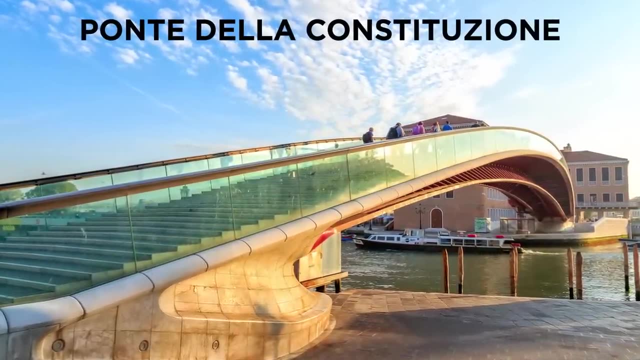 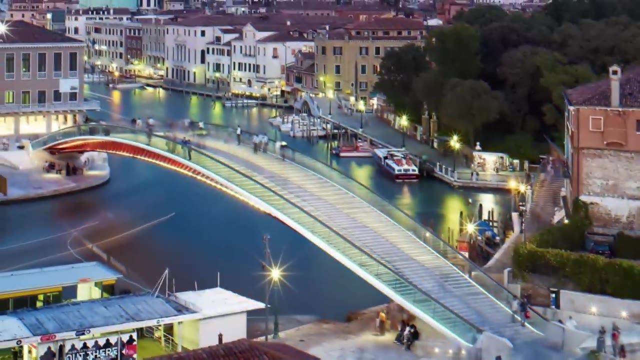 So Venetians were expecting something breathtaking for their upcoming bridge, But this was the result of Santiago's hard work. The Ponte della Costituzione, or Constitution Bridge: Stark, simple and bold. Citizens were pleased with the bridge's elegant, curved design and striking. 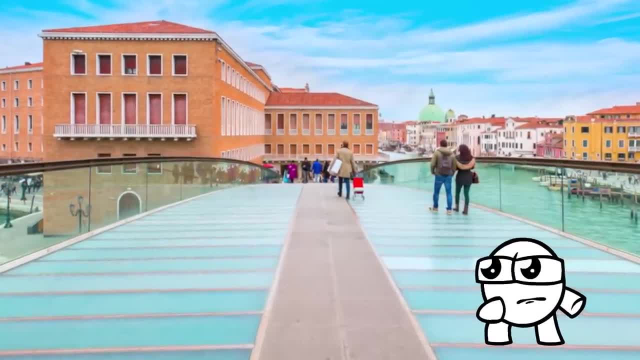 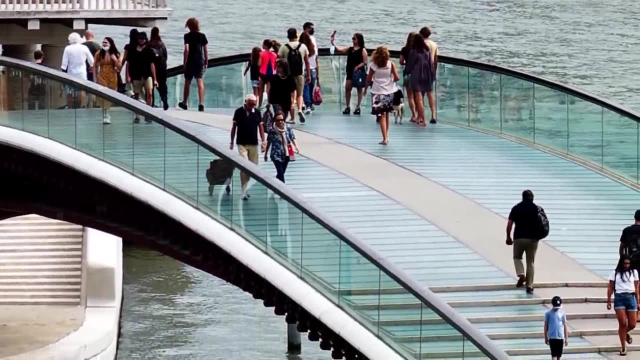 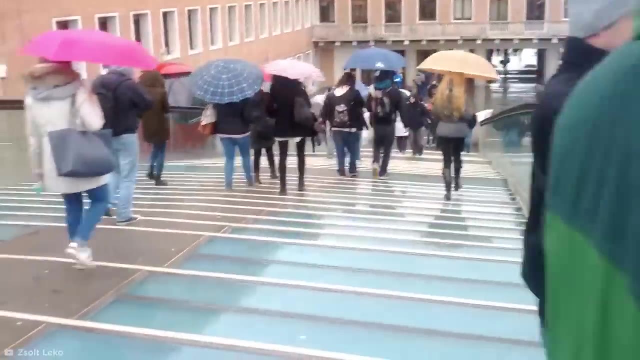 translucency, But there was something these Venetians were blind to. You see, to get that see-through, look just right, Santiago had primarily constructed the bridge out of glass. Why is this a problem? Well, Venice experiences around 32 inches of rain a year. 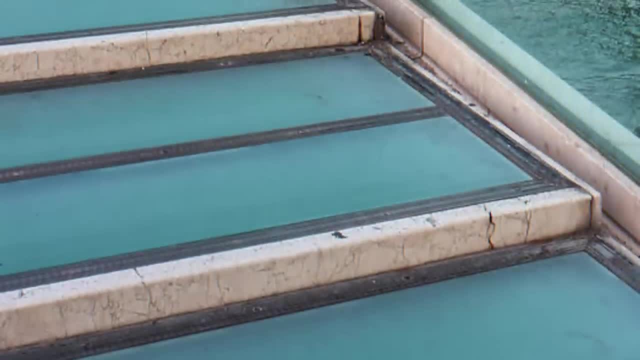 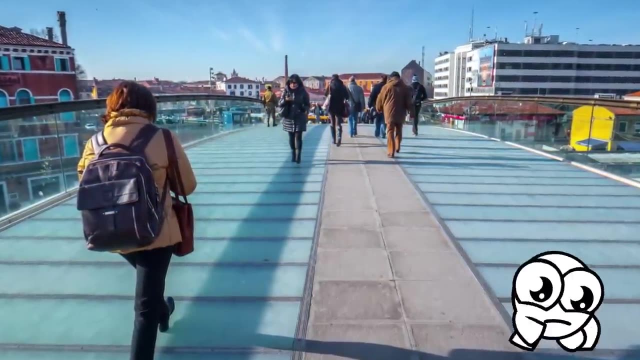 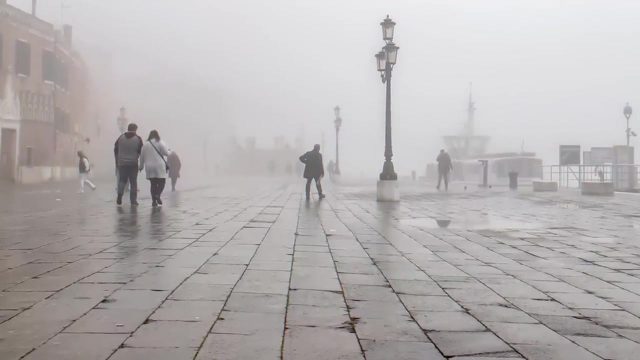 distributed pretty evenly across the months, And glass is a notoriously slippery material when wet. This made Constitution Bridge fairly treacherous to cross all year round, But in winter it was a death trap. In addition to receiving a lot of fog in the winter, the rain that fell 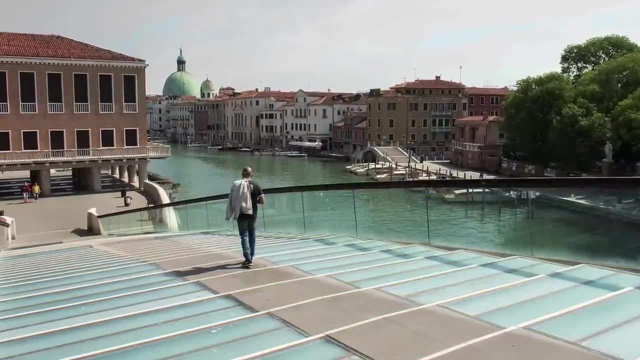 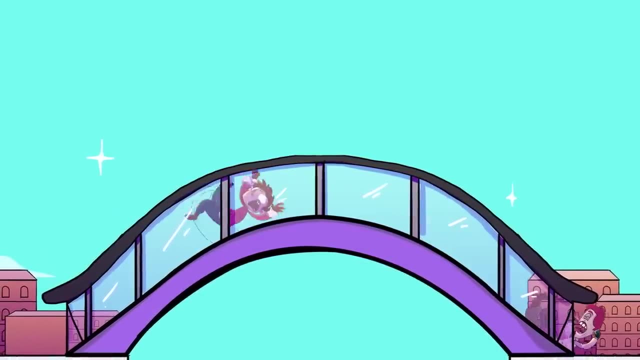 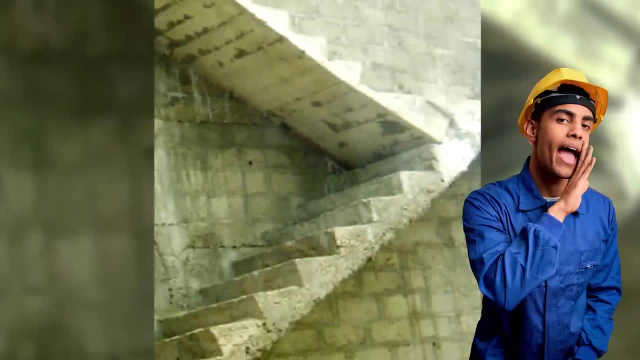 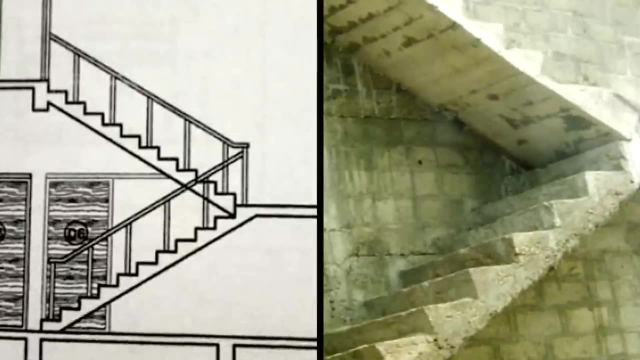 the bridge was a dead end. So the bridge was a dead end. So the bridge was a dead end. So orders. In this case, maybe the contractors got stiffed on the pay and decided to teach their client a lesson. You don't like these, boss? Well, we followed the blueprints you gave us. 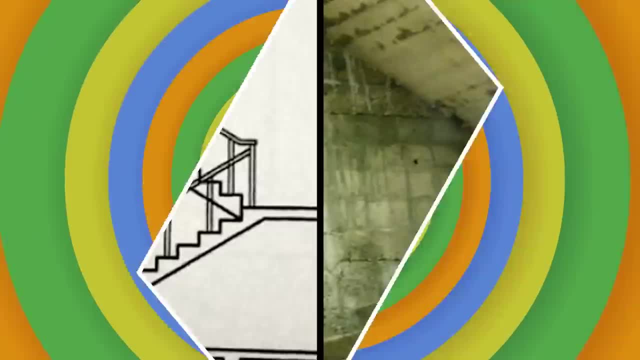 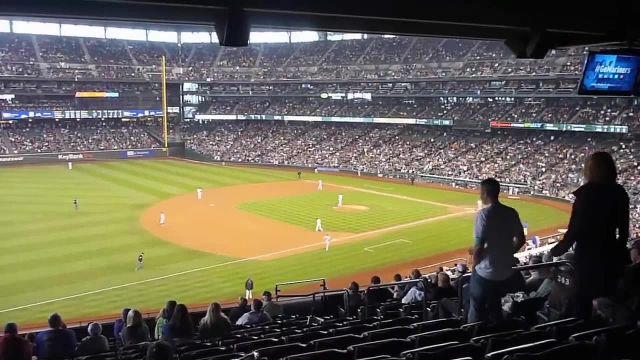 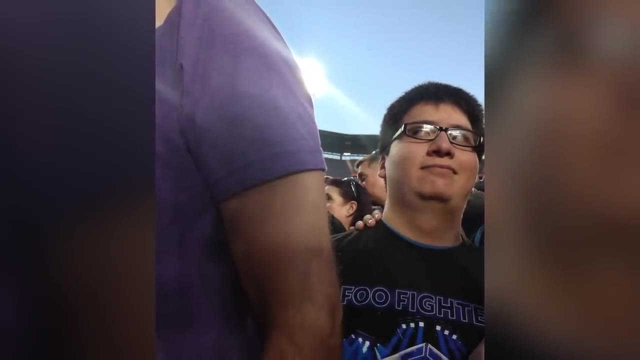 exactly. so what's the problem? The Edge of Your Seat. We've all lived through the indignity of excitedly sitting down at a sports ball event only to realize you're seated behind a giant that completely obstructs your view. It happens, but it's something the stadium can't really control. What they can control, however, 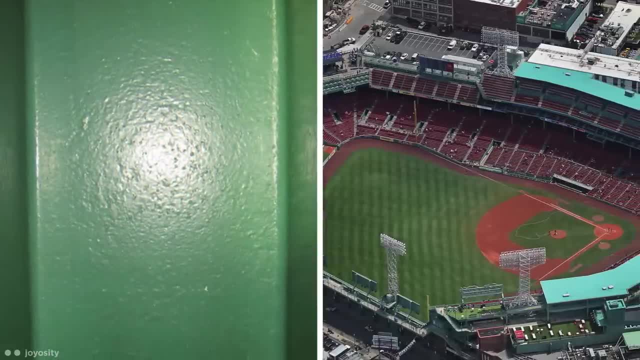 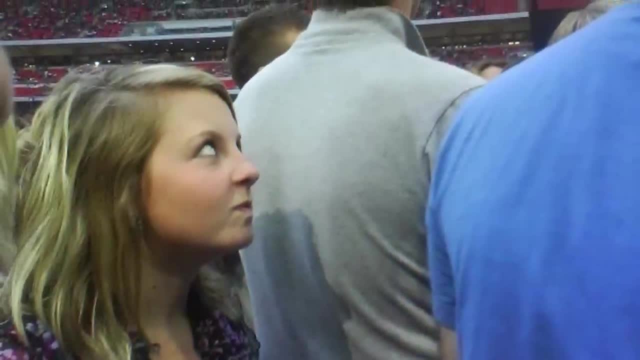 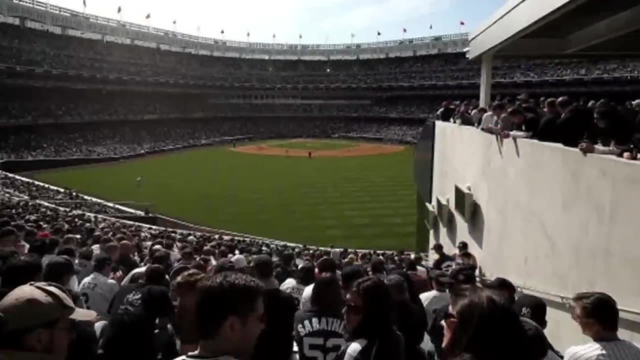 are seats like this in Fenway Park Stadium, where the fan's view is completely obscured by a pillar. Yeah, suddenly being sat behind Lurch doesn't seem like such a problem, does it? Well, how about this one in Yankee Stadium, where half of your field view is obscured by a raised? 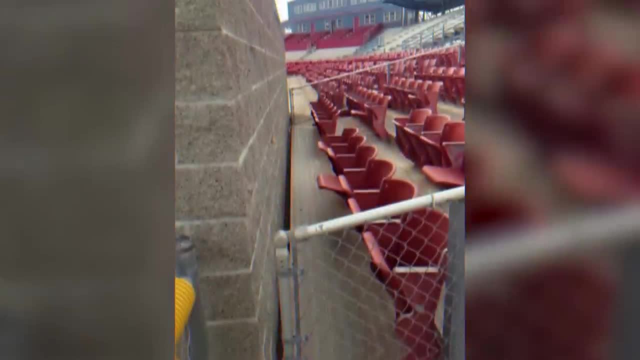 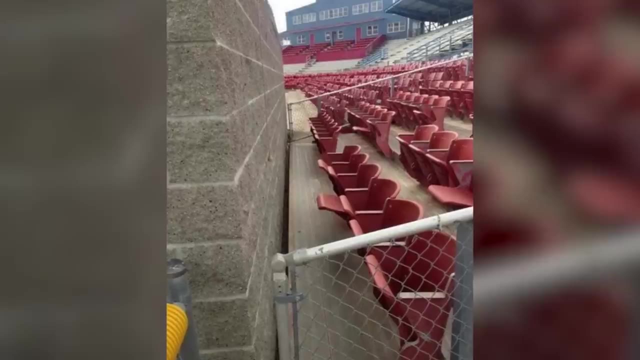 platform. Talk about a class divide. Finally, there are the Z-seats, And uh, I don't know what to say here. Maybe these seats were okay for a family of giraffes out at a ball game, but other than that, how do you explain them even existing? 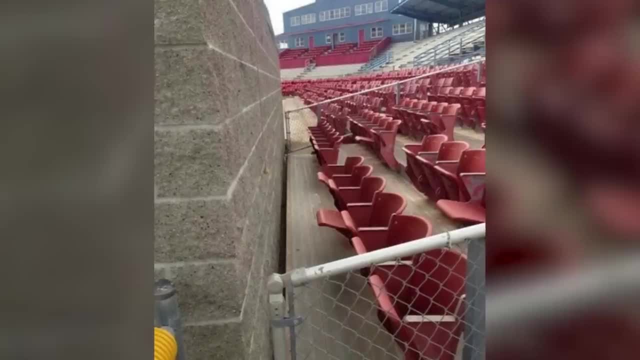 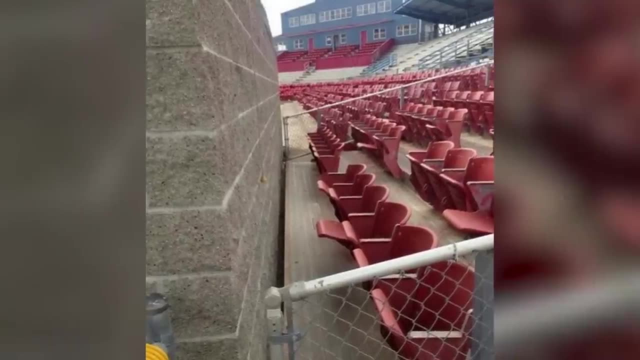 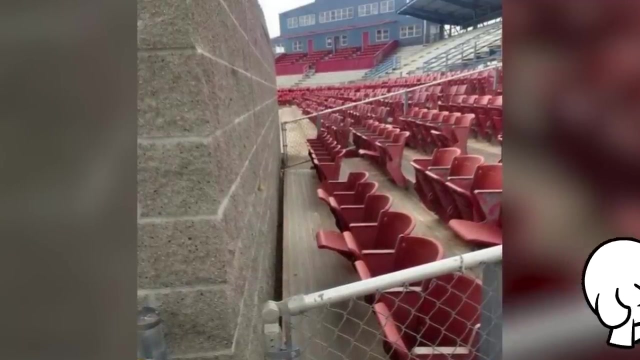 Well, many sports fans theorize that seats like these exist solely so stadiums can advertise a higher seating capacity than they actually have. No one is supposed to end up in these seats, but sometimes computers make mistakes and people are probably not. Well, that does it. From now on, I'm not going to a sports game without my trusty periscope. 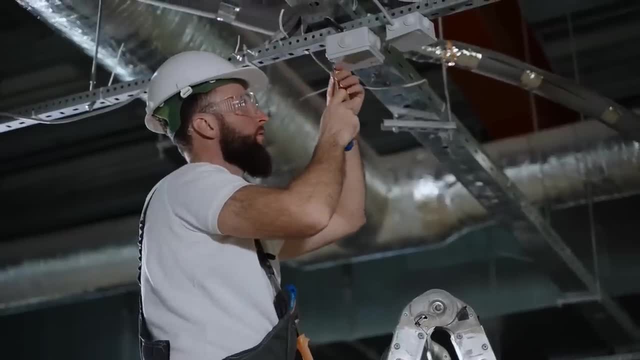 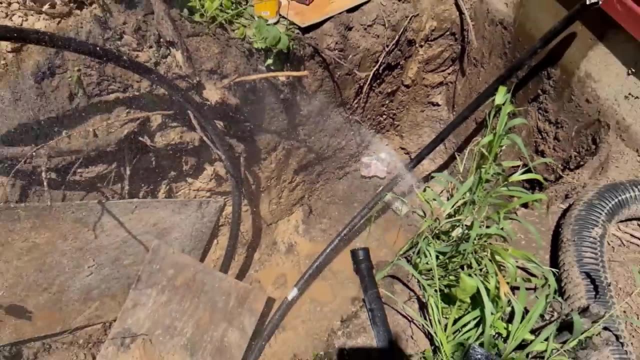 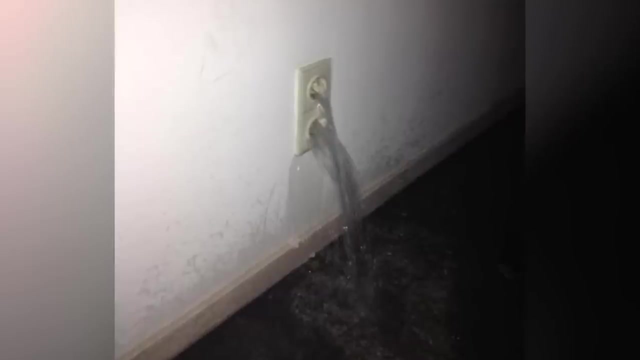 Sprung a Leak. Pipes and electrical wires in a house are a lot like our own bones and arteries And, just like us, they can break down if you don't look after them. Case in point, take a peek at this electrical socket that appears to have um sprung a leak. 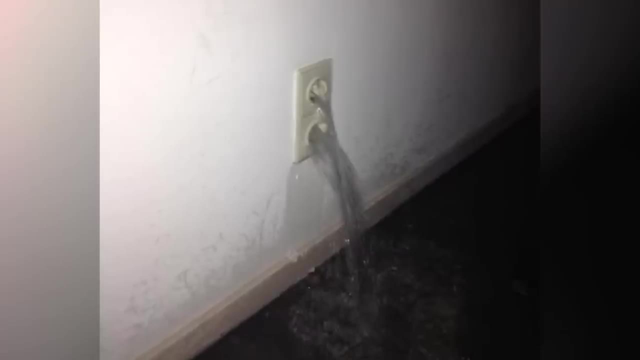 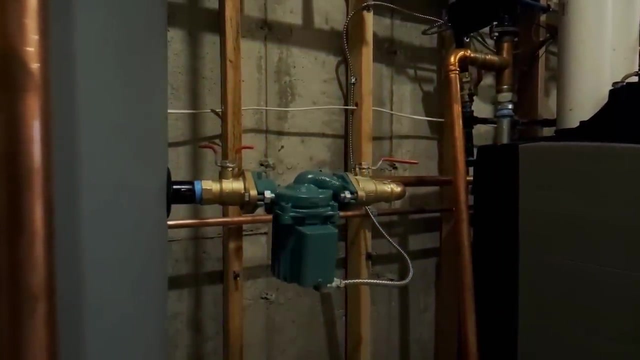 Wait what? How did that happen? Well, as crazy as it looks, it's actually a more common issue than you might think. You see, houses tend to be filled with pressurized pipes which help water get from one area of your 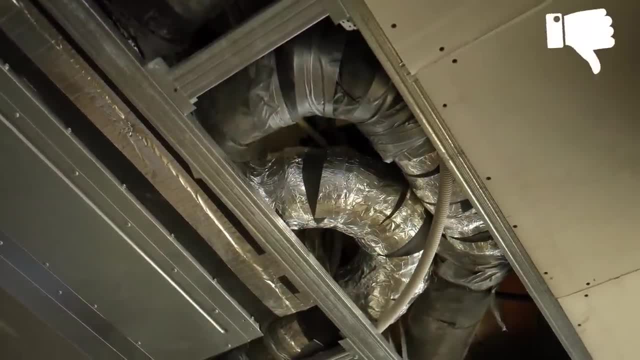 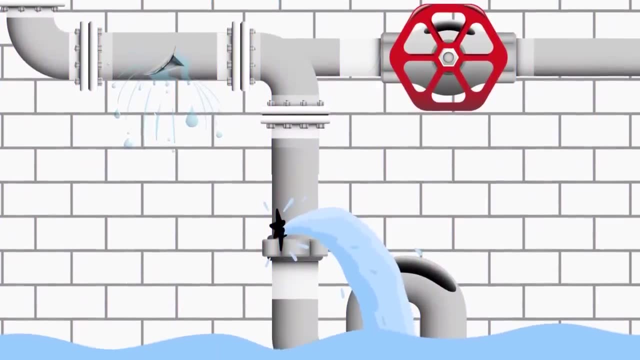 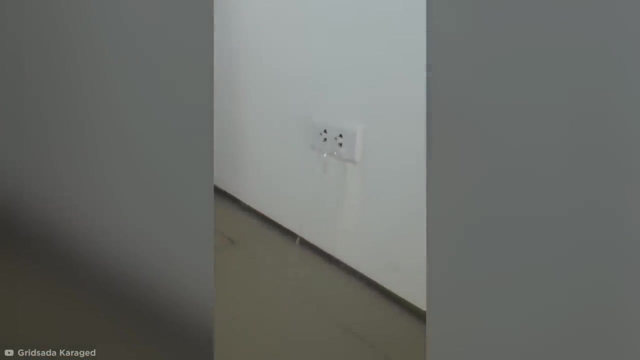 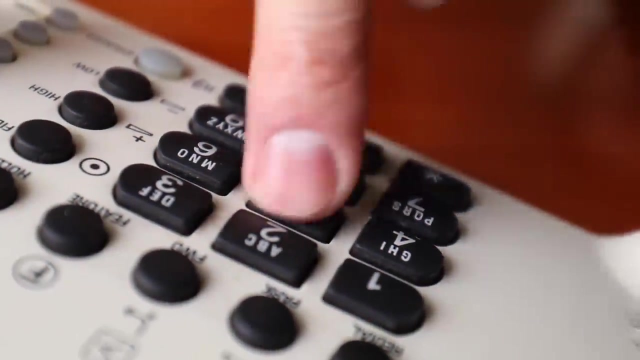 home to another. Sometimes, if these pipes are improperly installed or just worn down, they can crack. This leads to water leaking and pooling up inside your walls, And if you have a loose power outlet, creating an indoor waterfall. If this happens to you, turn off the main water valve in the building and call a plumber as soon as. 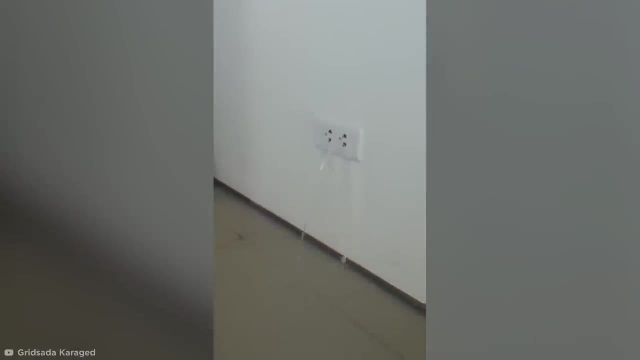 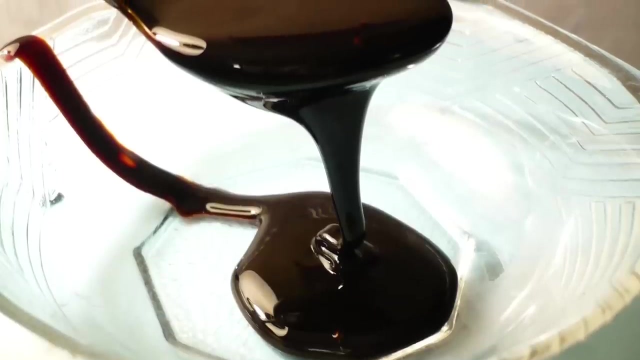 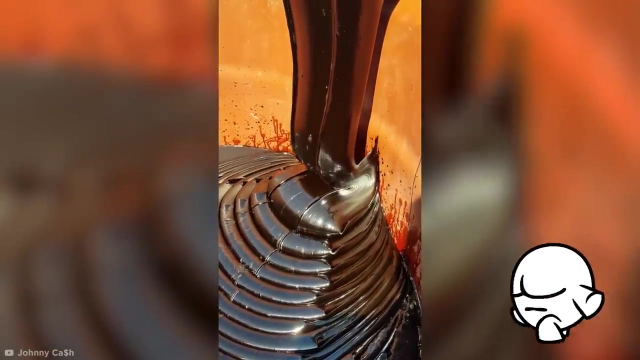 possible And no matter how bored you get, don't plug in your phone. Slow Burn. Molasses is a thick, sticky, dark brown substance known for its sweetness and extremely slow pouring speed. Yeah, if you've ever heard the phrase. 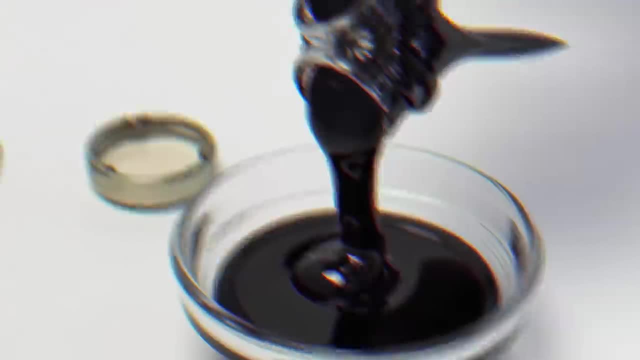 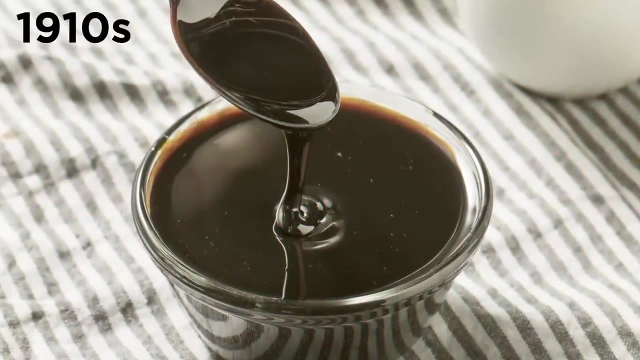 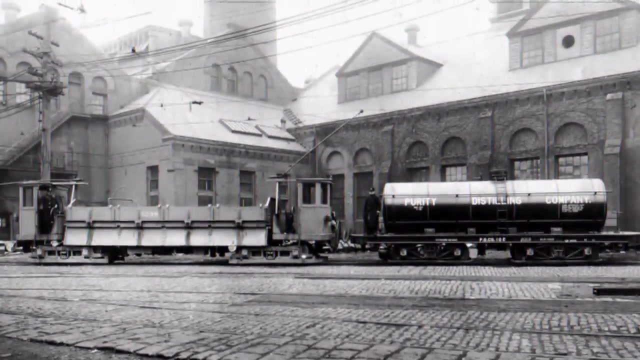 slow as molasses. this is why, In addition to being sickly sweet, however, did you know that molasses can also be deadly? In the 1910s, molasses was experiencing a boom in popularity as a cheap alternative to sugar. During this time, the Purity Distilling Company opened up. 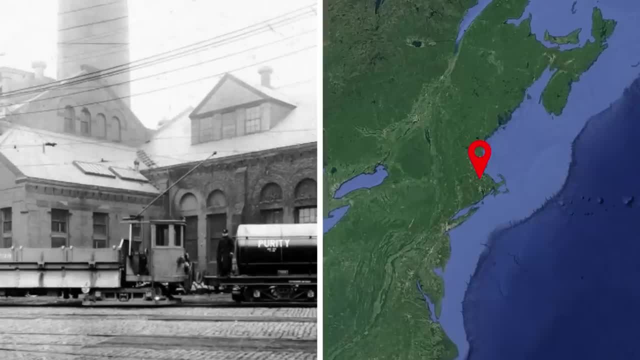 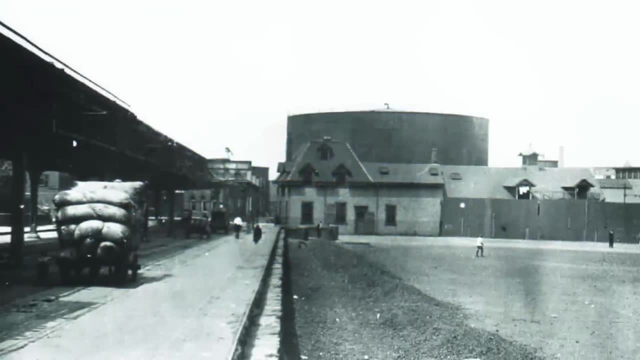 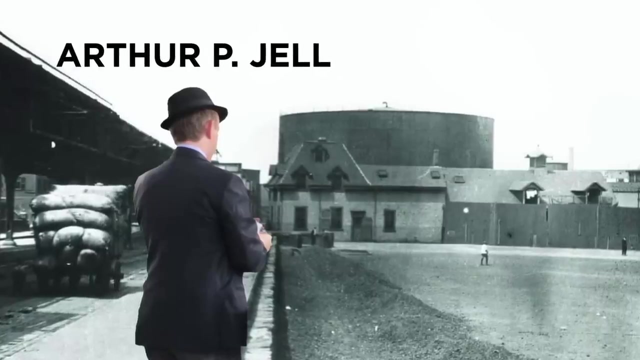 a molasses processing plant in Boston, Massachusetts, and their safety precautions were a little lacking, to say the least. As the company expanded, they quickly built a new distillery whose construction was overseen by a man named Arthur P Gell, But Gell was a financial advisor. 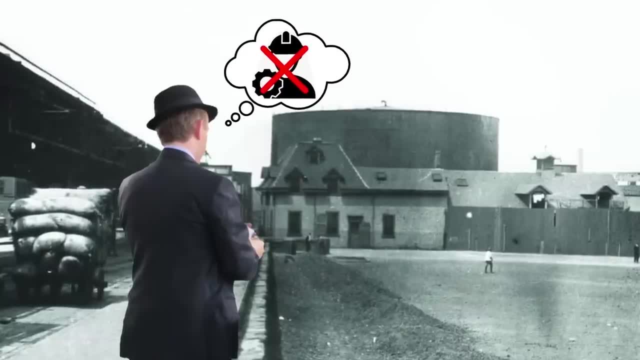 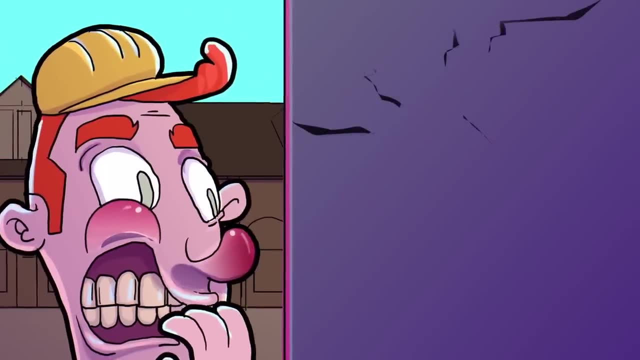 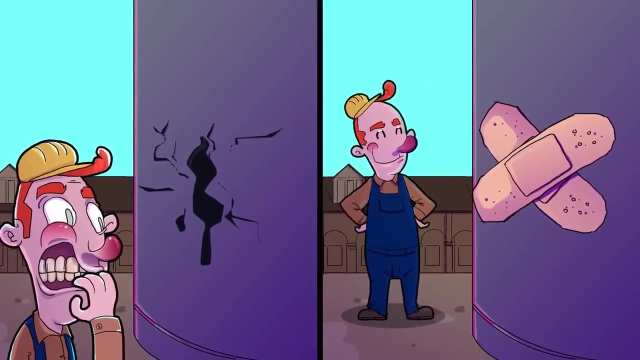 and had no experience in engineering, But he was cheaper than a trained engineer. As you can probably tell, it didn't take long for one of the main tanks at the facility to spring a leak, Which was hastily patched up. However, as more and more cracks began to form the company. 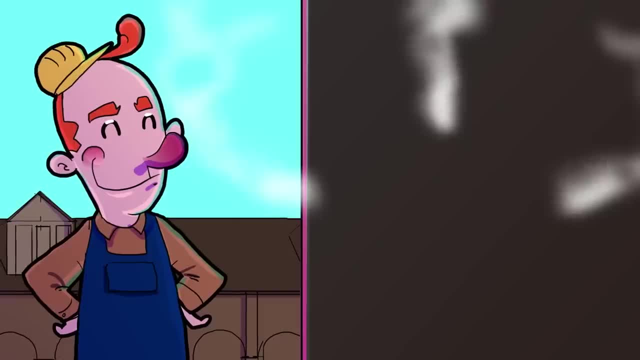 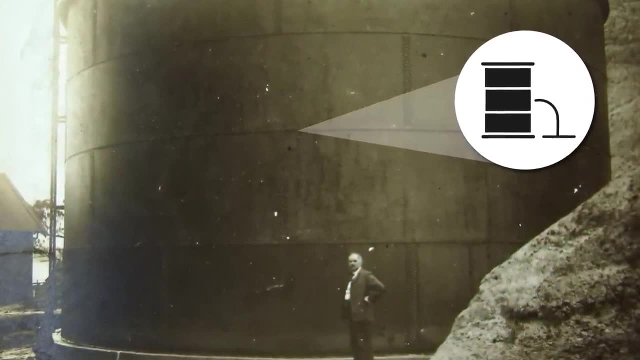 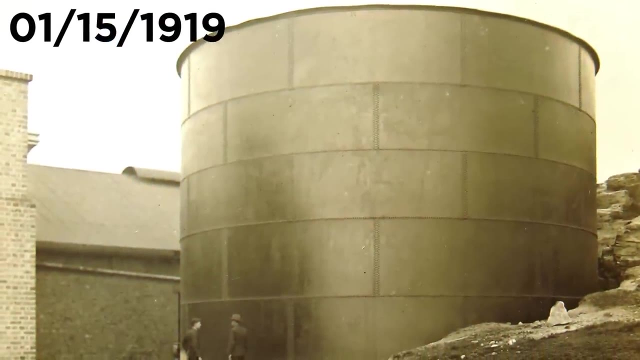 had the bright idea: why not just paint the tank a dark color? No really, they figured, if no one could tell the tank was leaking, then there was no real problem. Ingenious right? Well no, On January 15th 1919, the 50-foot-tall tank finally gave out letting. 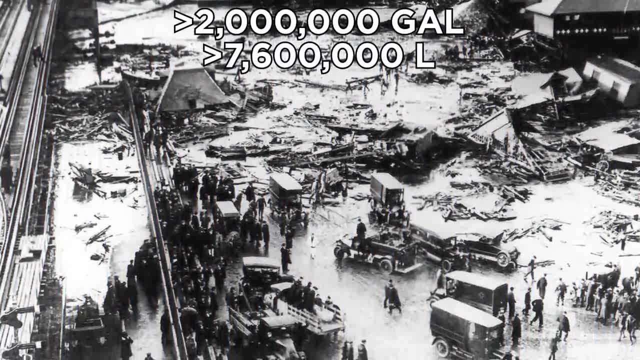 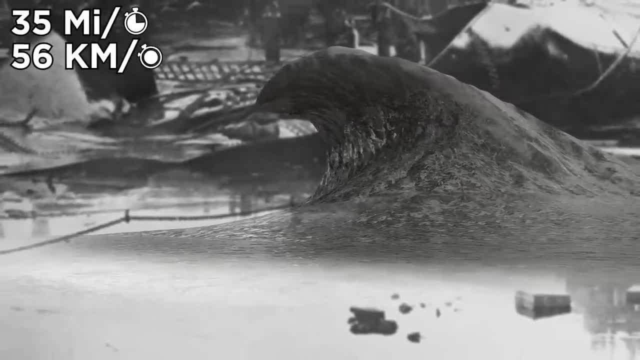 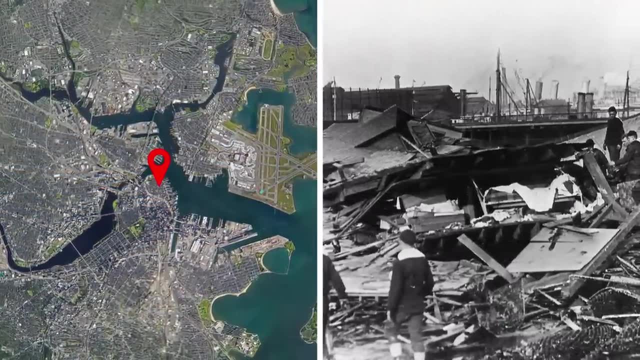 loose a landslide. It was a tank of over 2 million gallons of molasses. The wave was apparently 55 feet tall and traveled as fast as 35 miles per hour. As the tank was only 200 feet from the harbor, it caused huge damage to the city and ended up injuring 150 people. If you're. 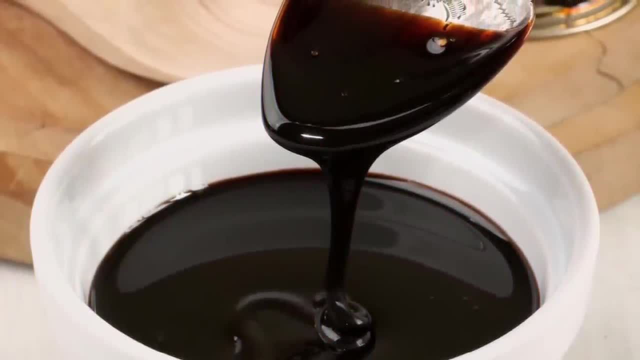 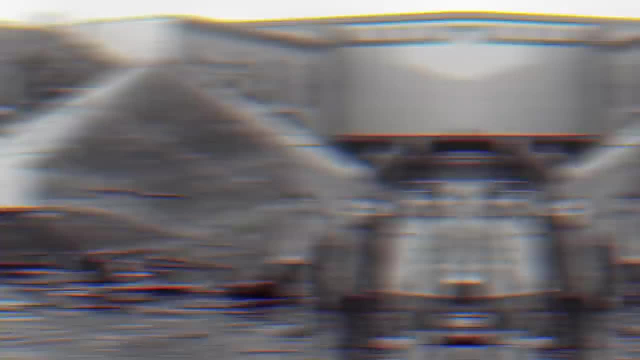 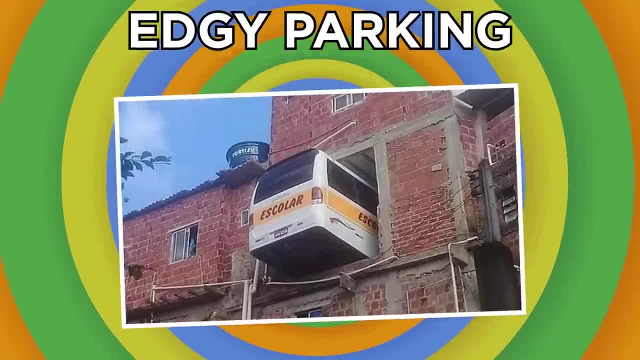 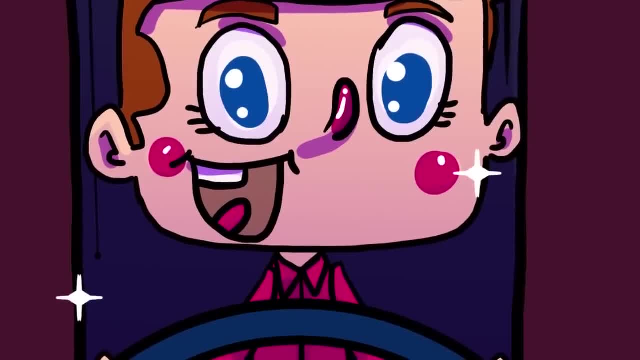 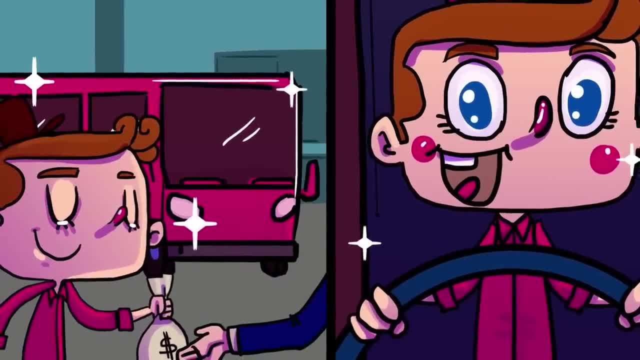 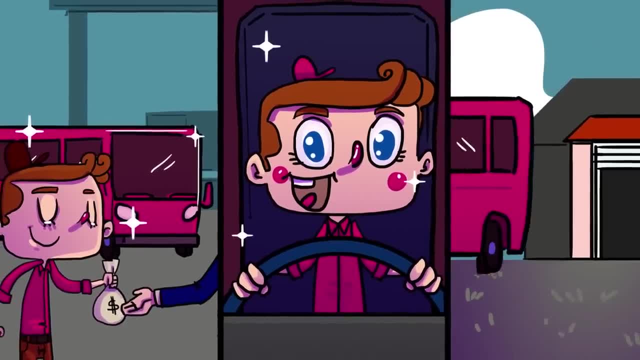 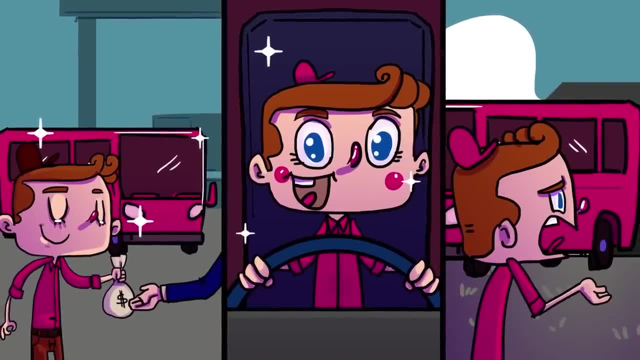 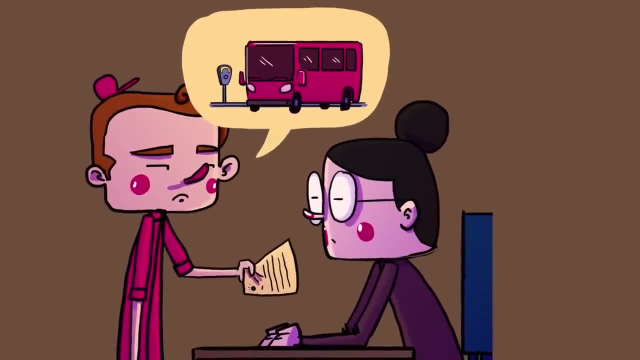 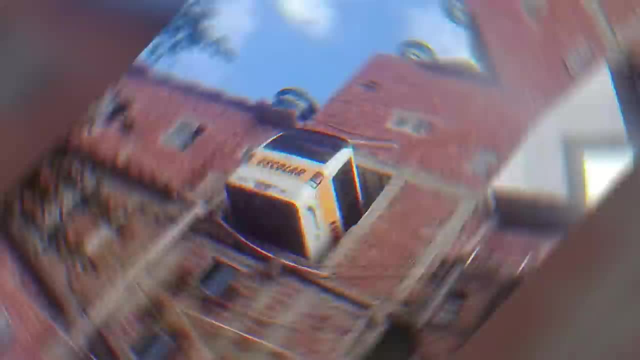 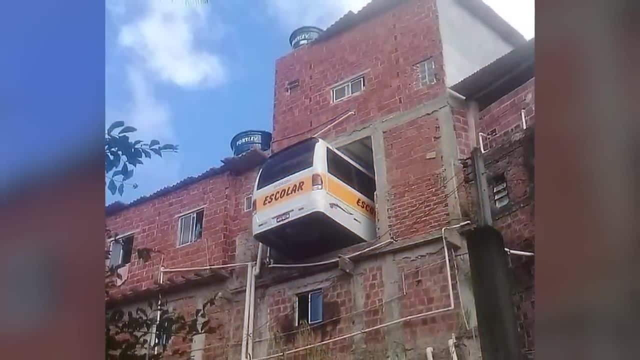 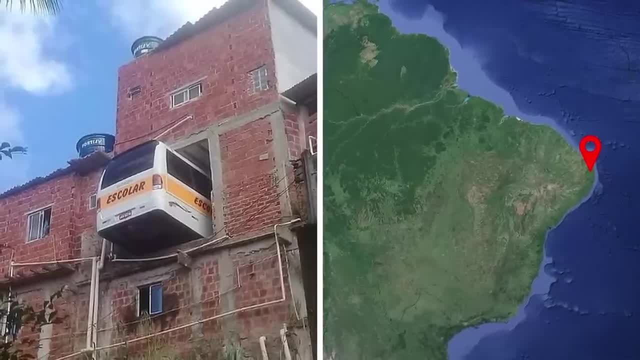 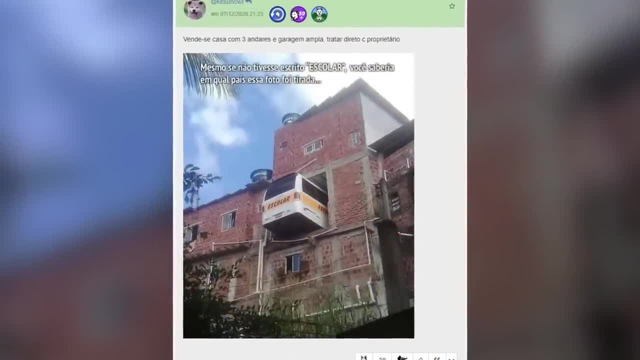 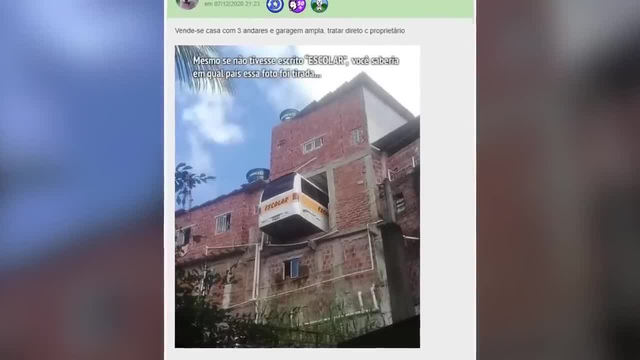 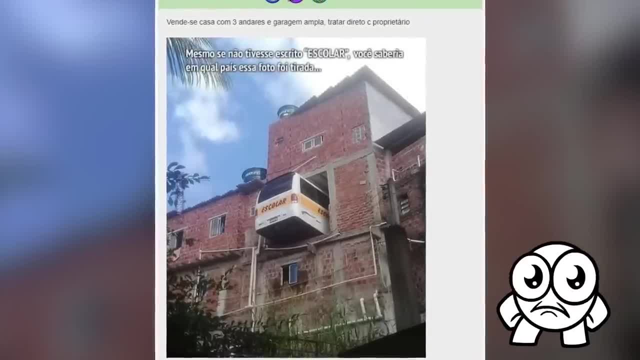 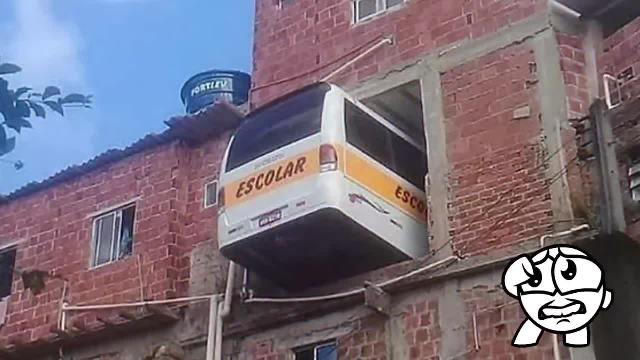 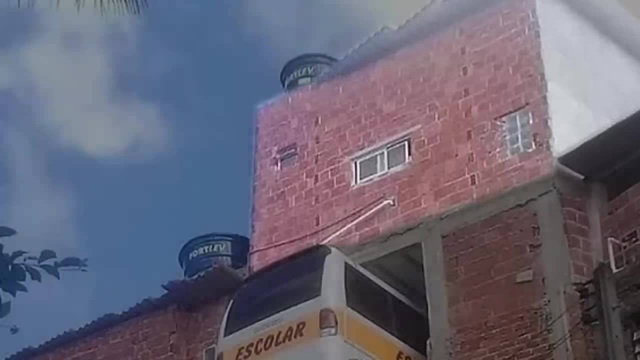 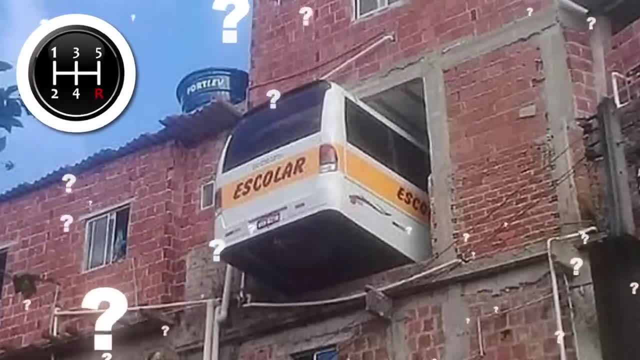 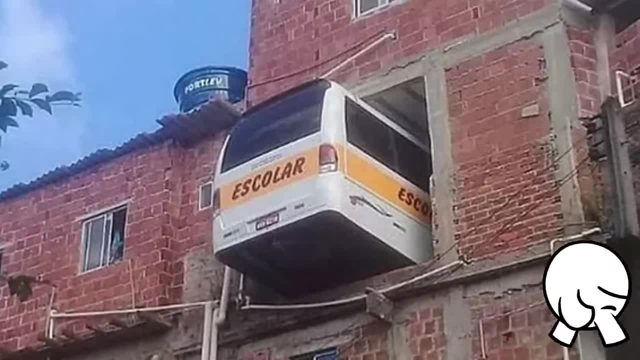 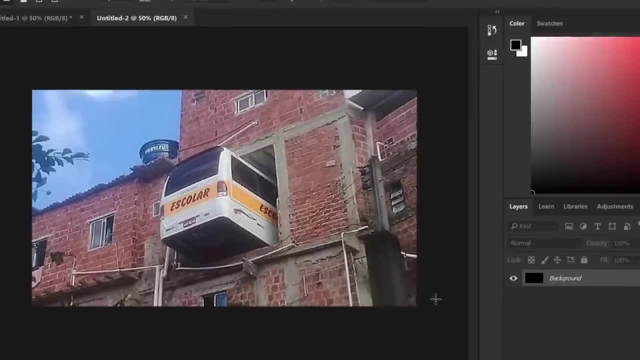 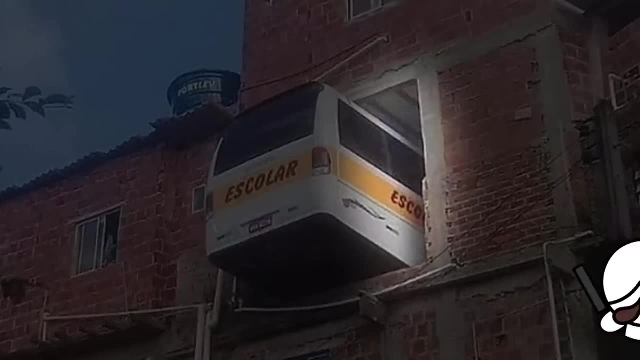 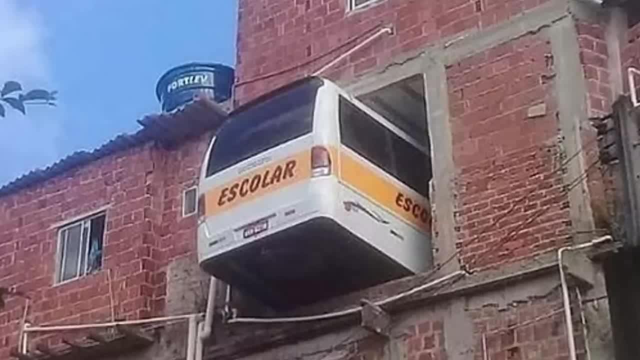 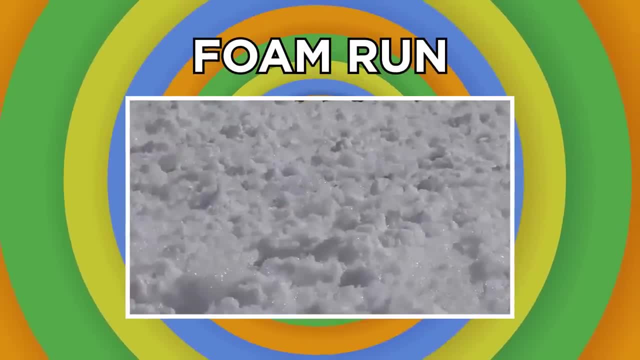 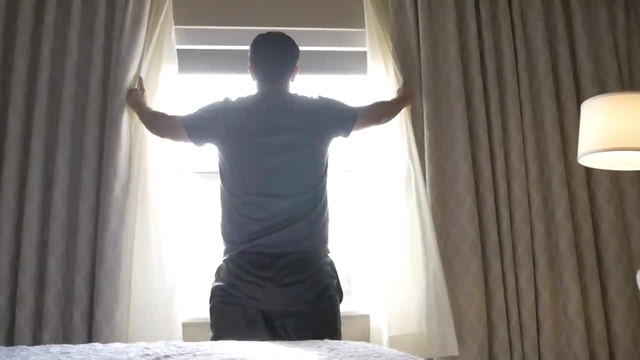 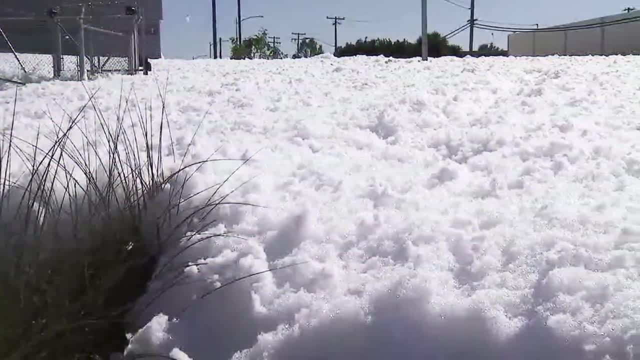 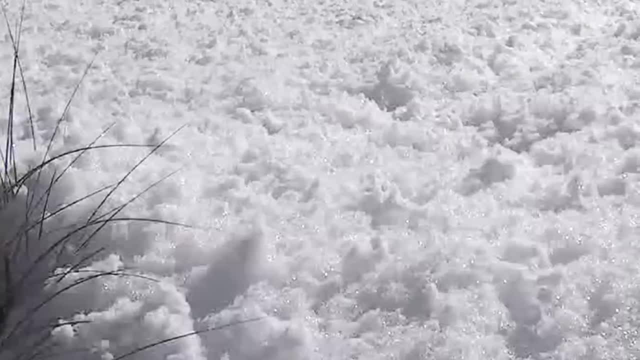 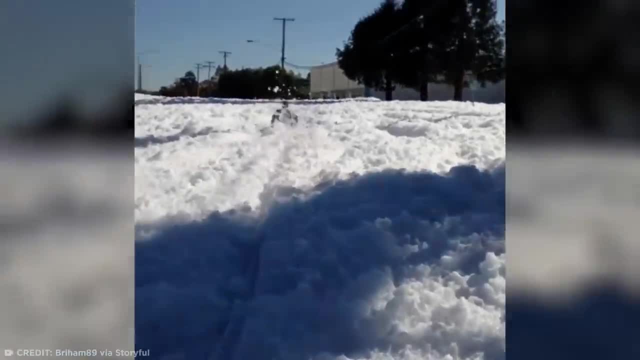 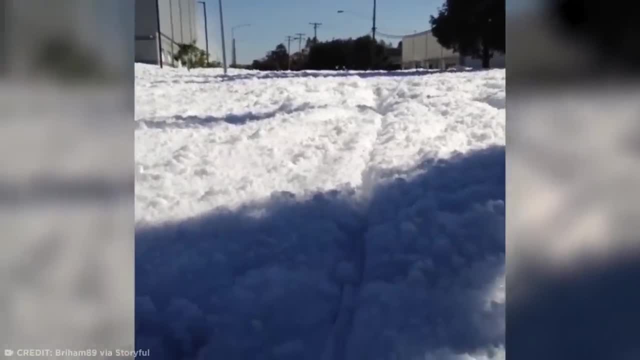 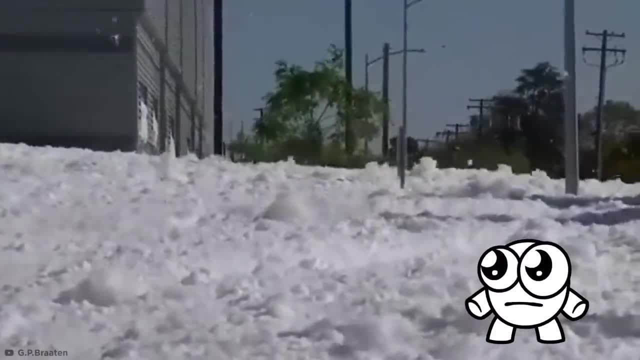 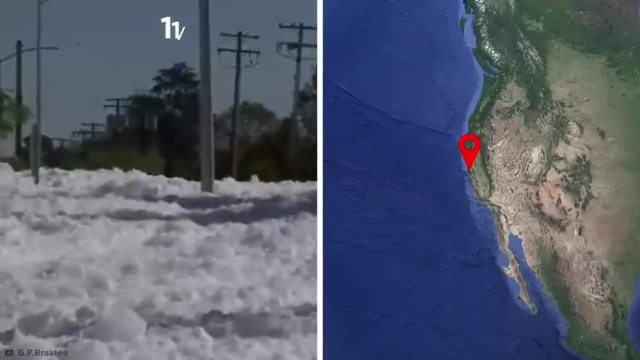 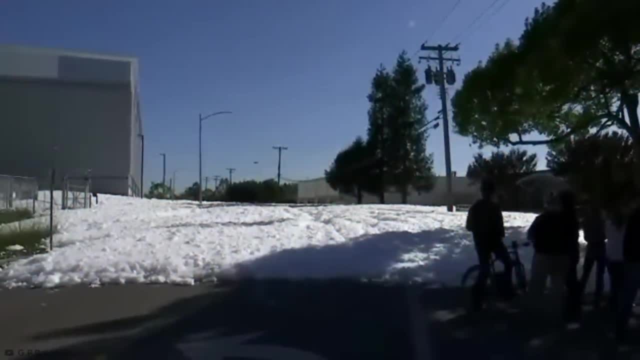 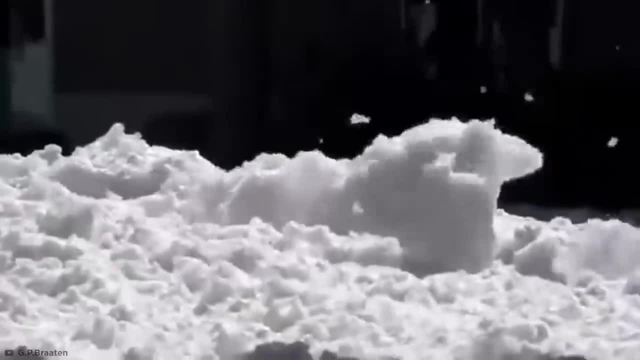 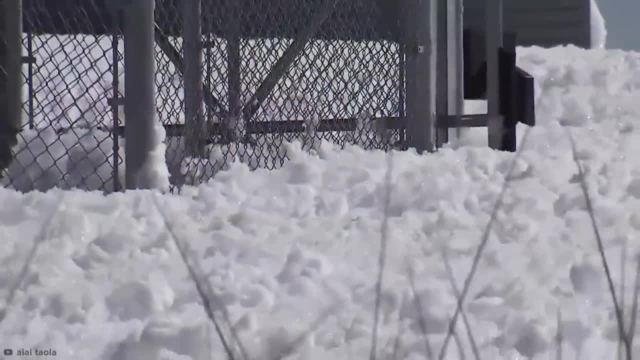 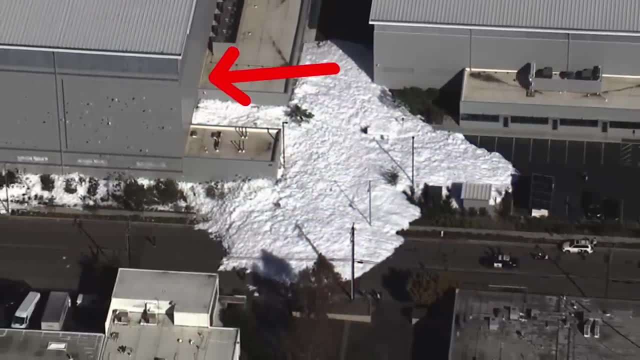 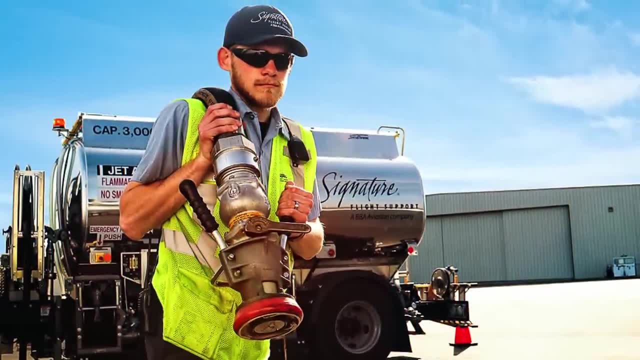 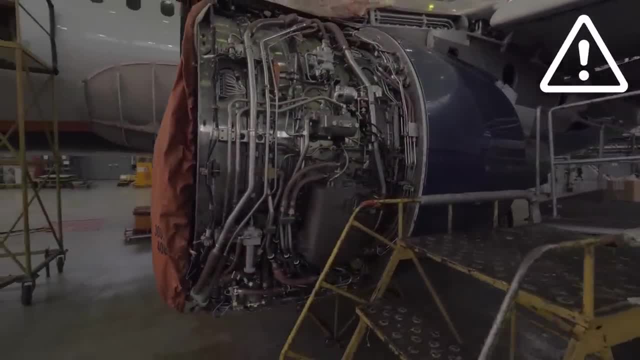 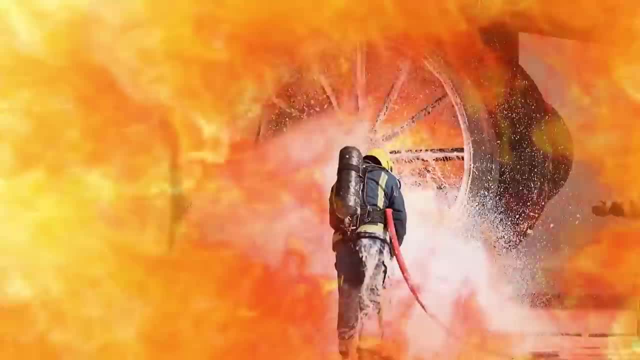 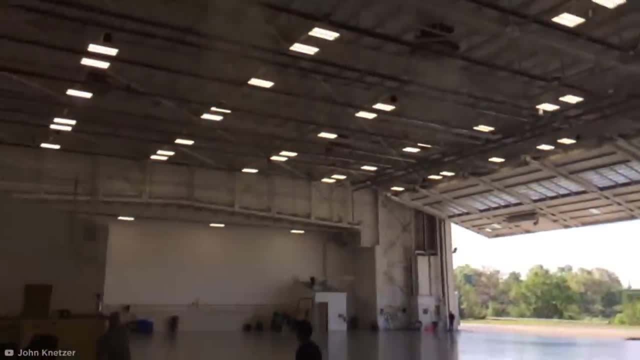 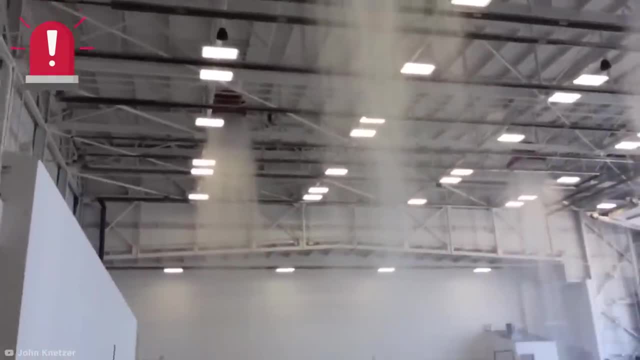 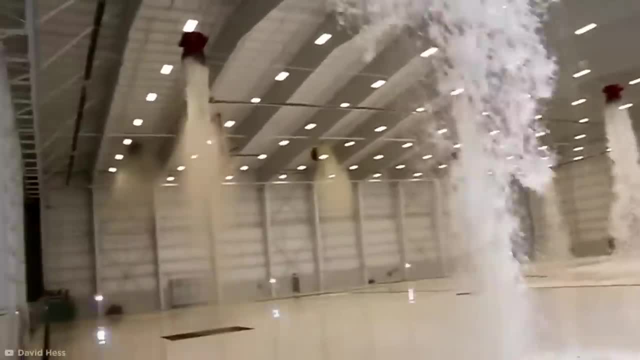 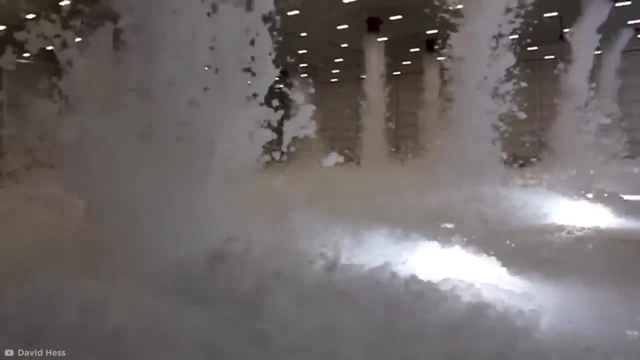 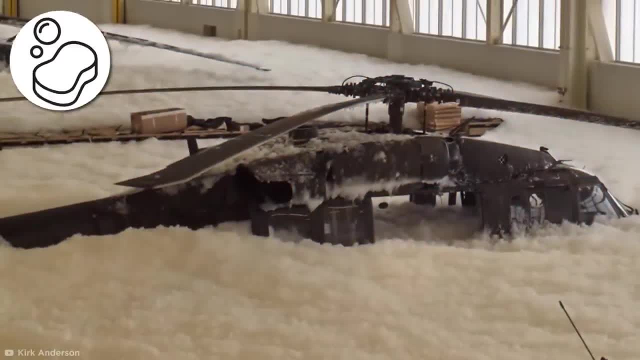 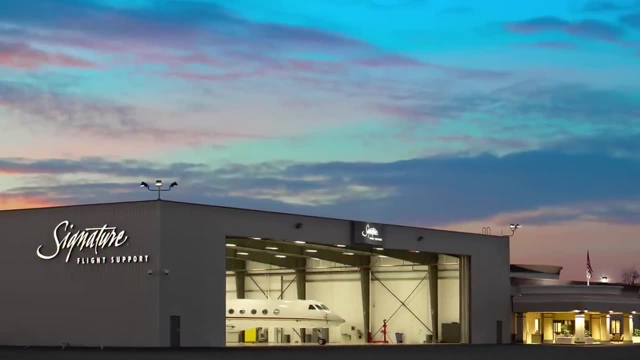 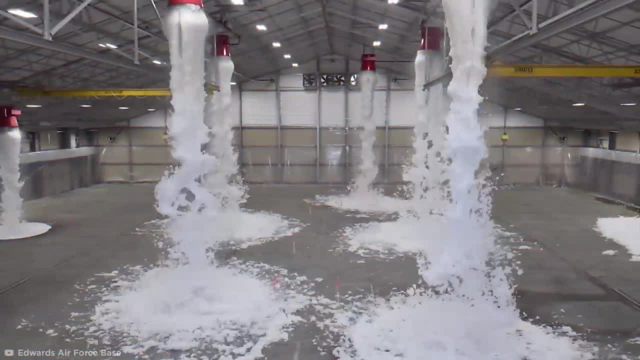 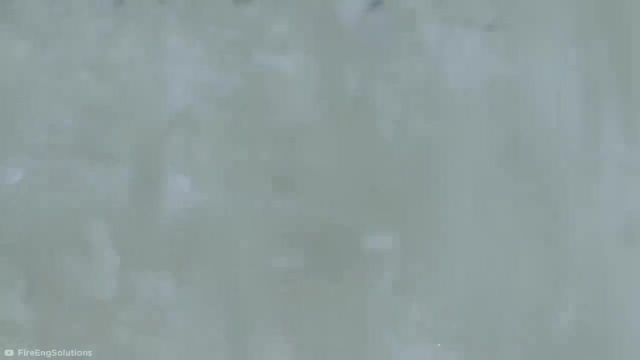 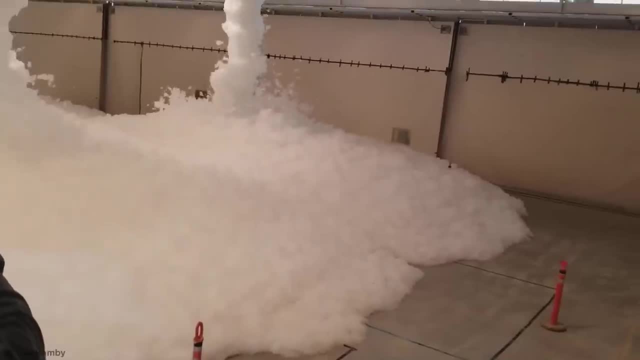 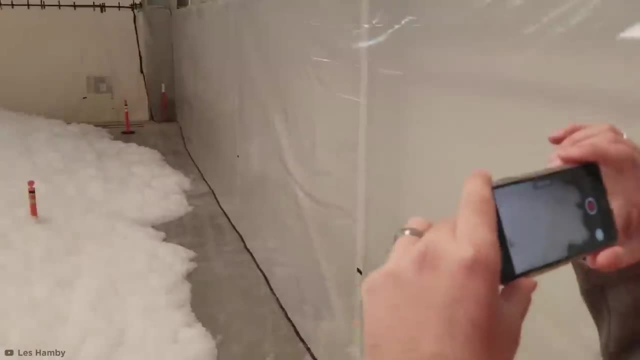 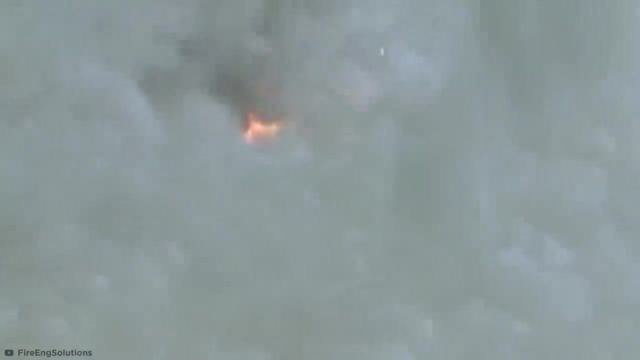 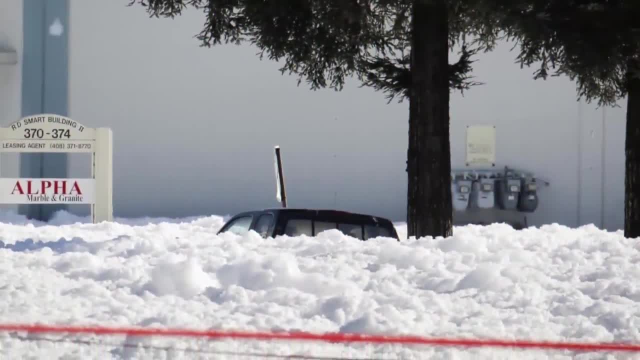 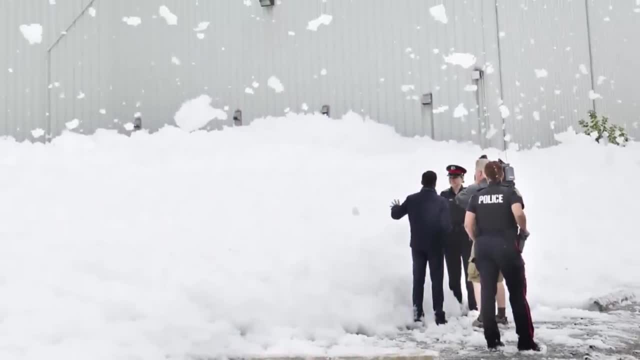 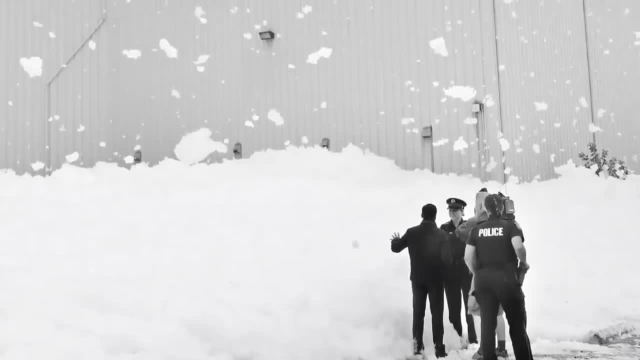 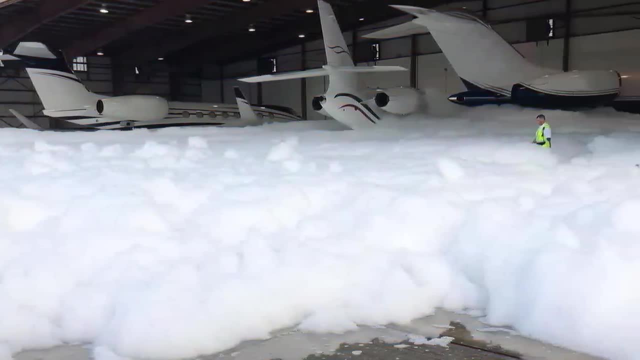 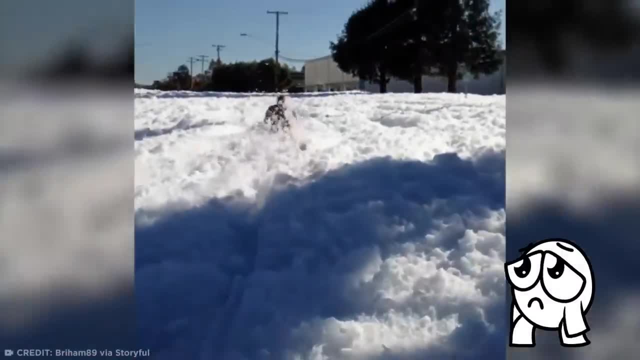 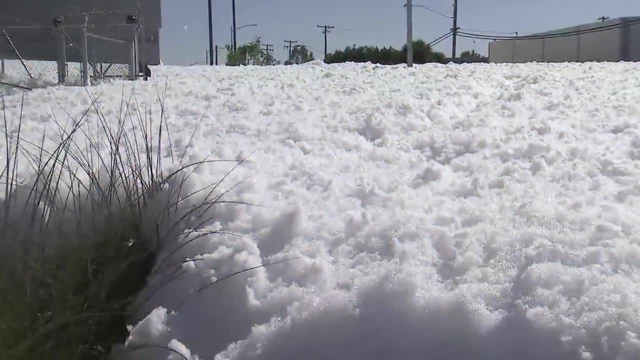 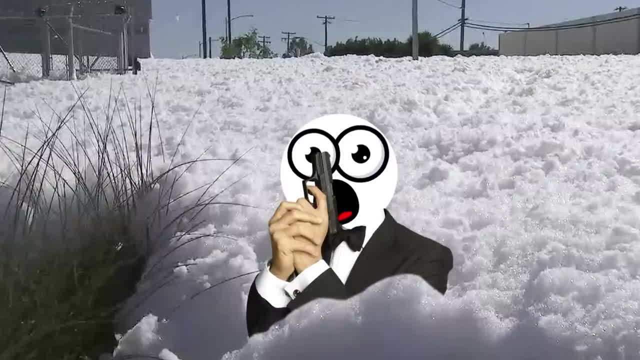 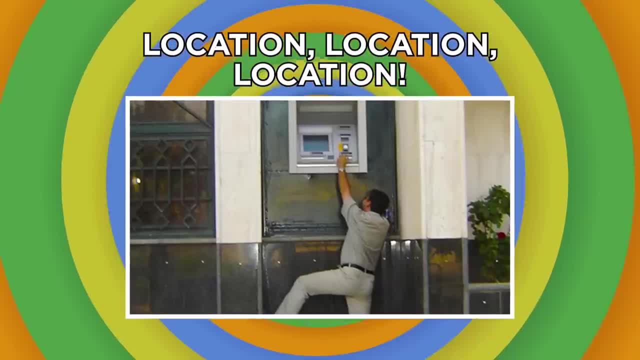 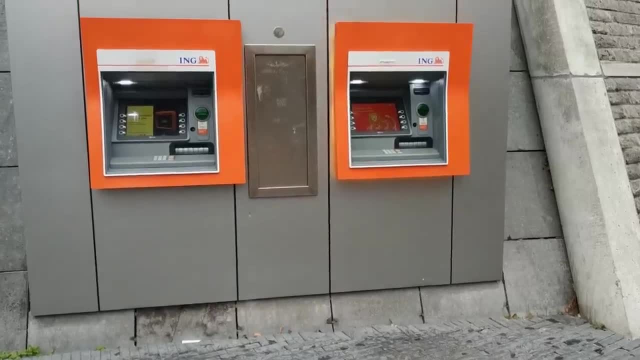 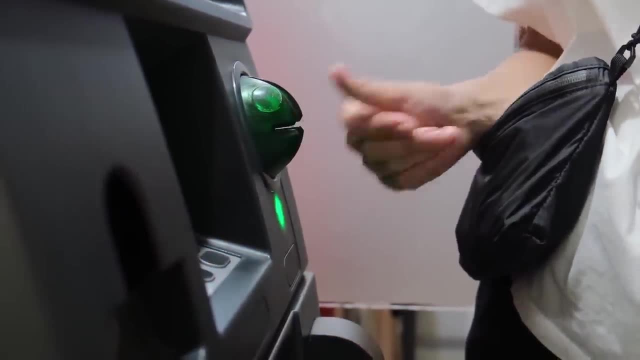 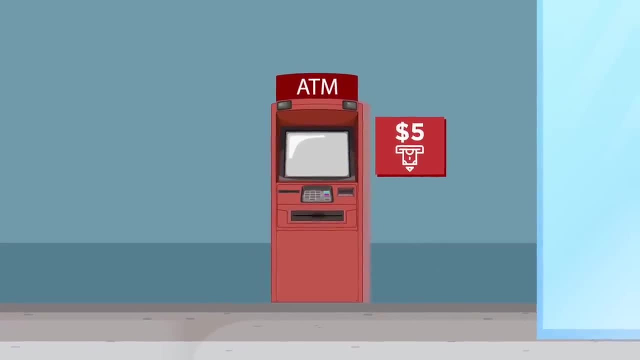 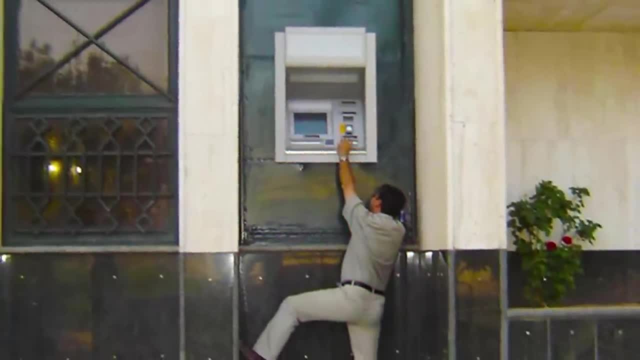 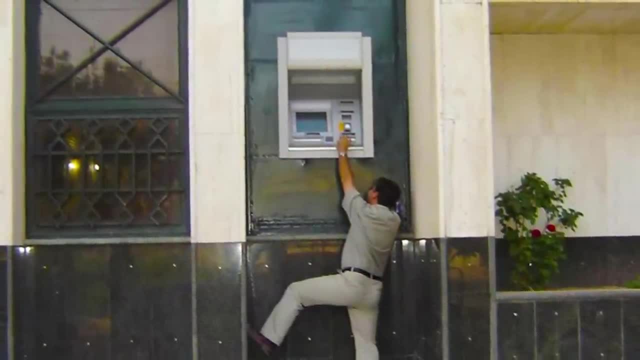 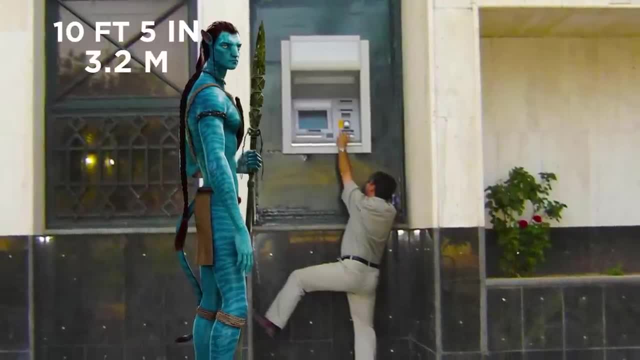 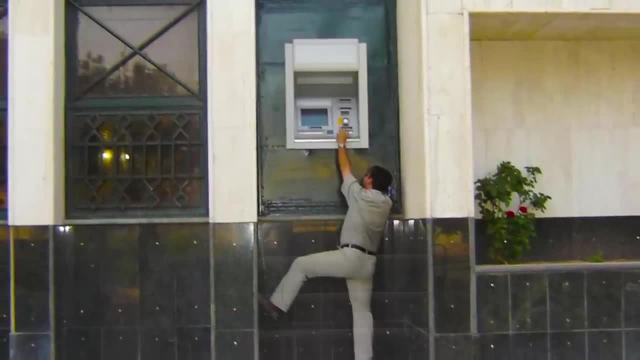 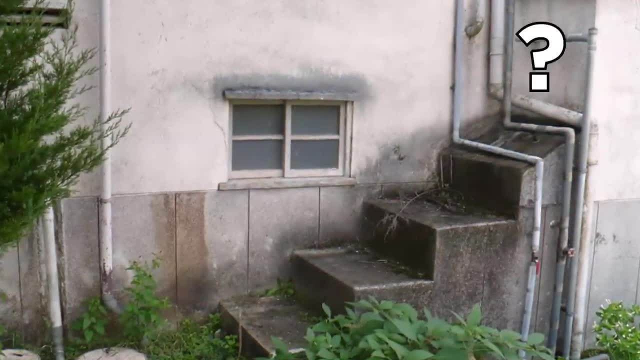 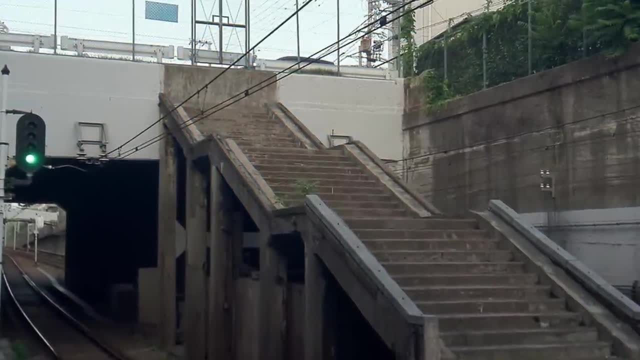 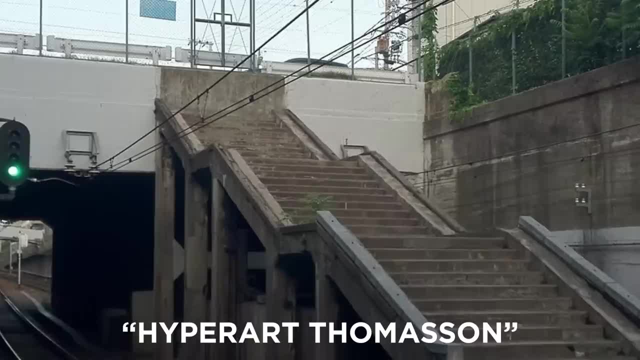 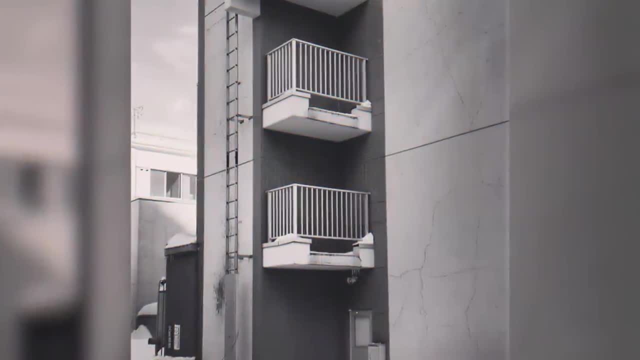 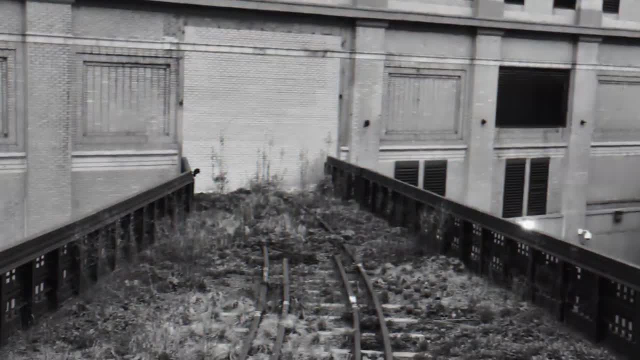